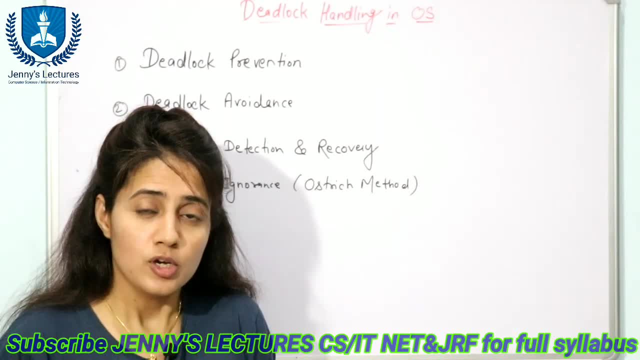 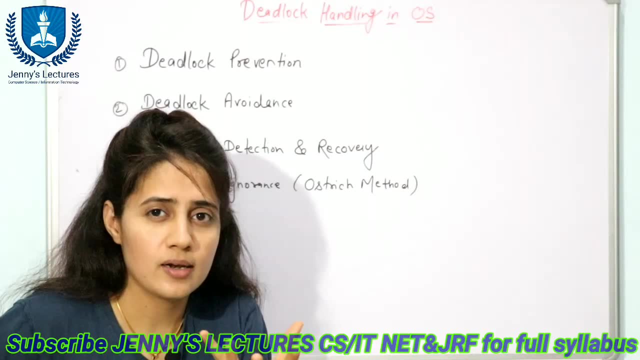 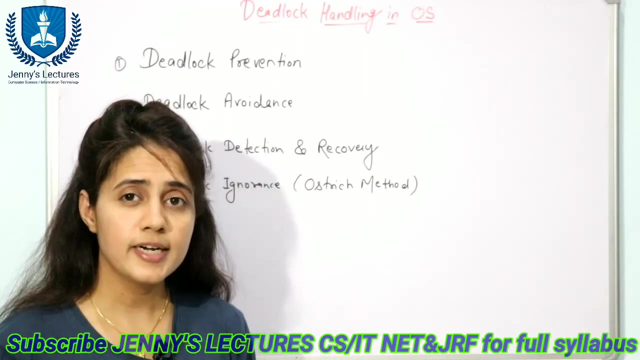 go to 35 marks. These are second category of students. So these, these students are just, they are just avoiding the failure. They don't want to perform well, but they just want to avoid the failure. so third category of student is: they'll not work hard, they'll not study. they think that. why should? 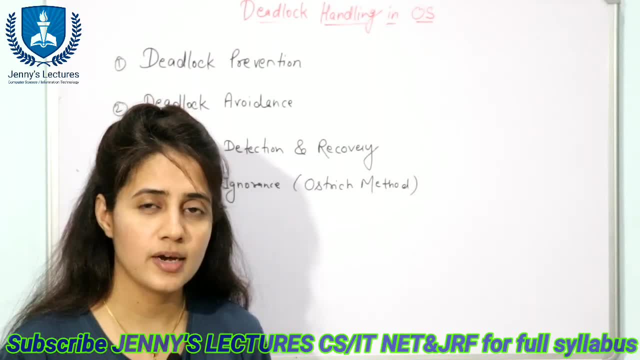 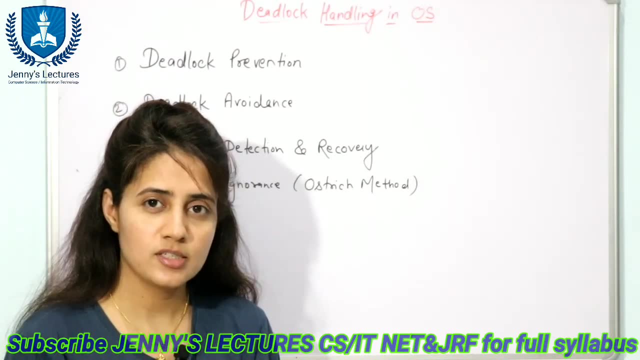 i study, maybe i might apply that tukka kind of thing and for first 10 questions i just mark a, and for next 10 question i just mark b and something like this. and maybe, maybe, uh, they can get 35 marks that cut off marks so they can get passed. so when, maybe at some time? 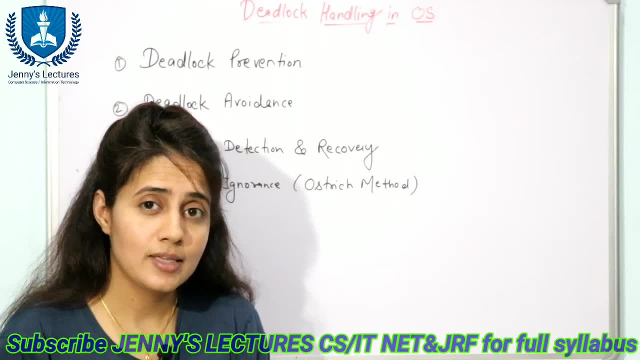 when result come. then they find, they find that they detect that they got less than 30 marks, less than 35 marks. so now, at that time they detect the problem and then they want to recover that problem. maybe they think that the next time will work hard and will get above 35 marks. fine, so till: 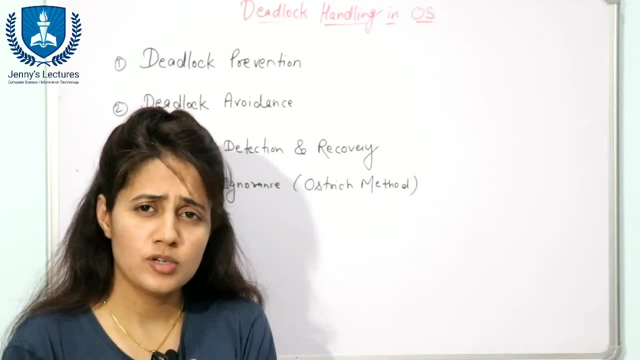 till the problem doesn't come. these kind of students are very cool. after problem comes, they detect the problem and they try to recover that problem. fine, now, next category of student is they. they just ignore the problem. it doesn't affect that they are. they are getting 35 marks. they are getting 30 marks. they are getting minus 30 marks. 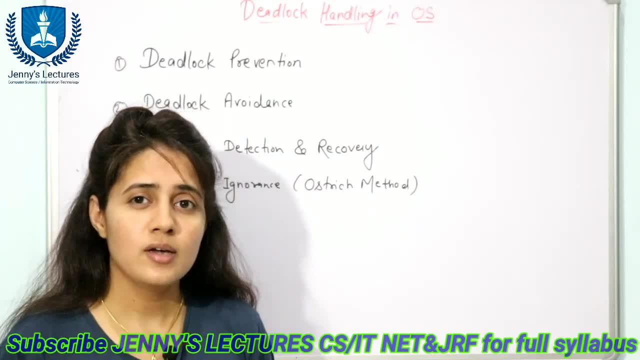 or they are getting maybe 80 marks. that is fine with them, so they are just ignoring the problem. it's something like that: if you think that there is a problem, then obviously there is a problem. if you think that there is no problem, then your mindset will be something like that. that, yeah. 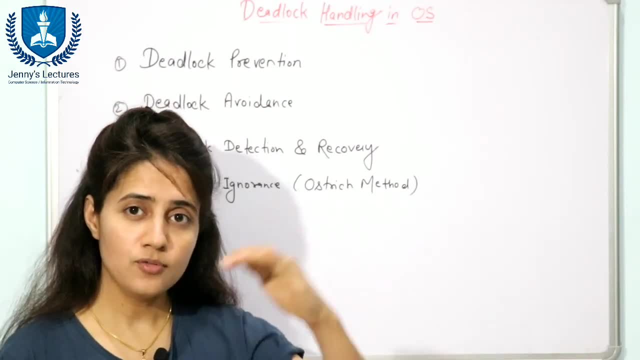 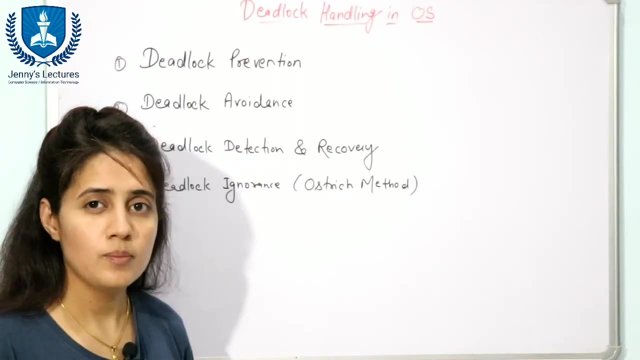 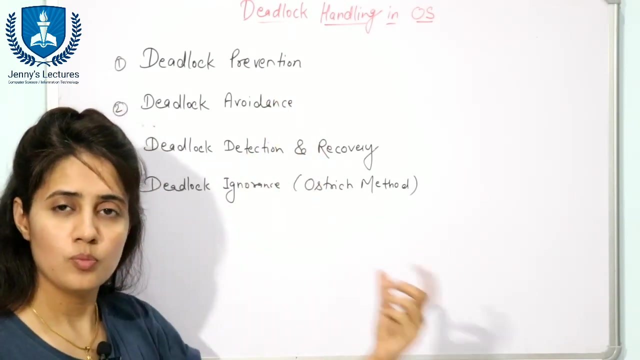 there is no problem and you are very cool. see, all the four category of students have solved the problem with their own method. so if you come to the terms of operating system, then here also we have these four kind of method to handle deadlock or problem. fine, now, first method is: 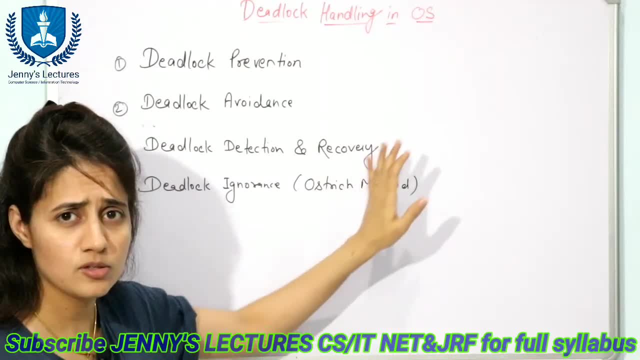 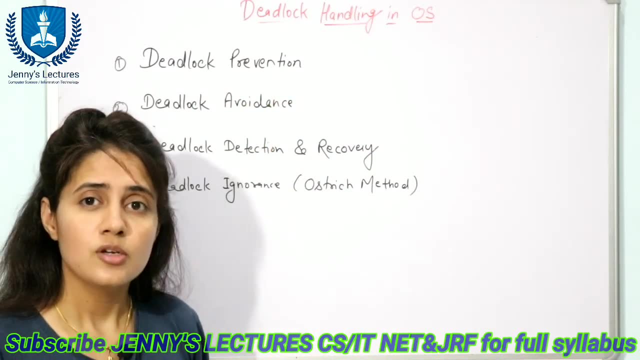 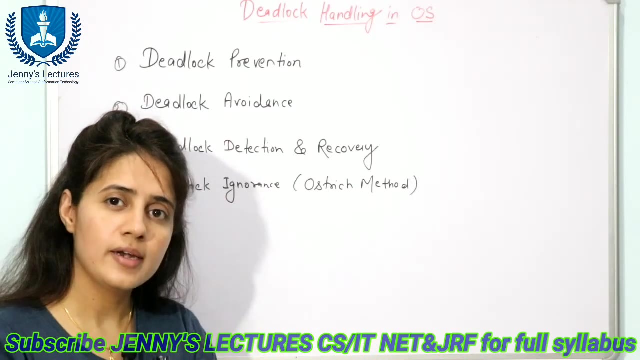 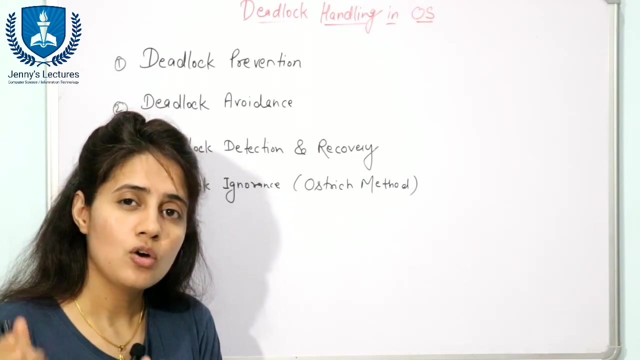 deadlock prevention. we can't say this method is best and this method is not good. see, it depends. we will discuss that thing also. first of all, see what is deadlock? prevention means prevent the deadlock from occurring. do something that deadlock will never occur, maybe using some techniques, apply some set of protocols such that a deadlock will never occur. 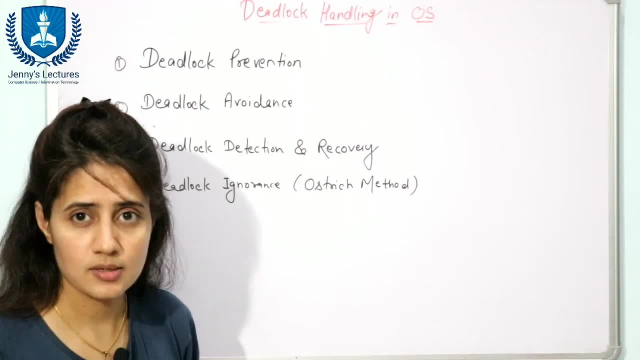 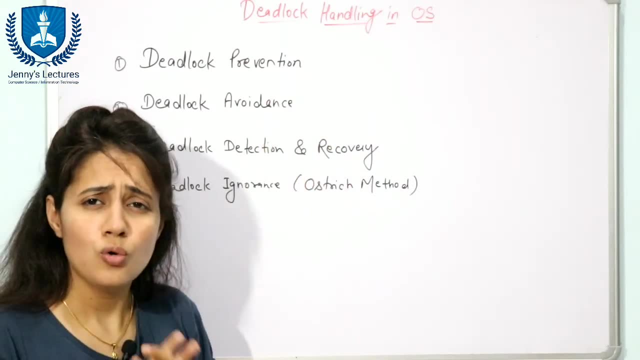 in the system. so obviously you can say that this one is best. if you prevent the deadlock from occurring, then obviously this is the best. but problem is that if you do something like that, even with this case, is what? lots of effort will be needed to write down the code. how to prevent. 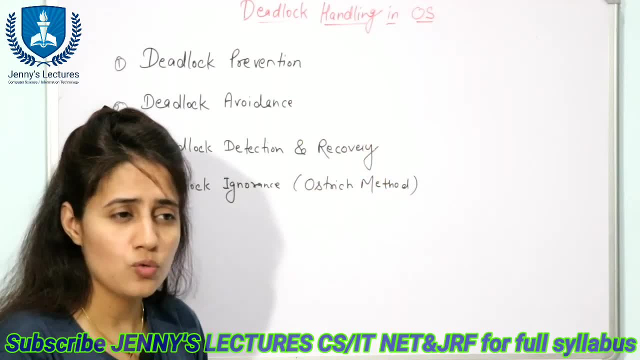 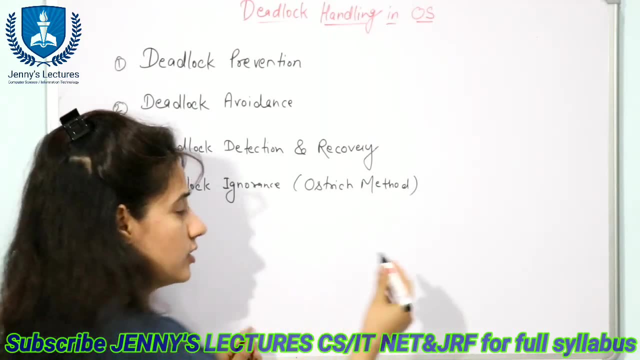 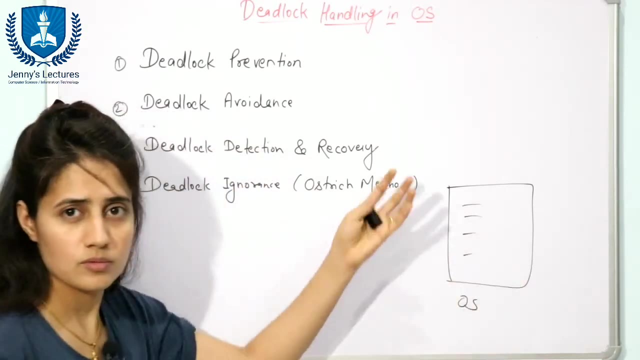 deadlock and obviously that cost would be very much cost in the sense, like in case of time complexity, in case of space complexity, and if you add one more functionality to operating system, see and see, suppose this one is your operating system, this one is code for your operating system having some functionalities, and if you write one more code to 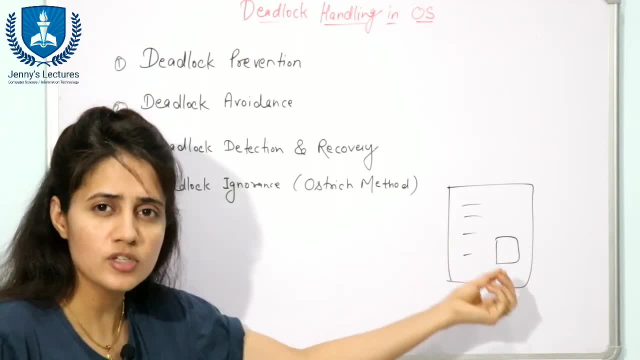 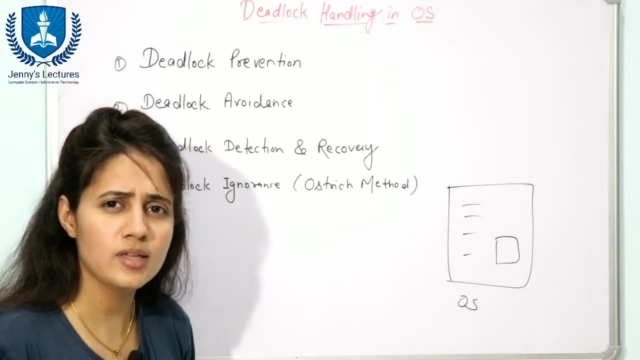 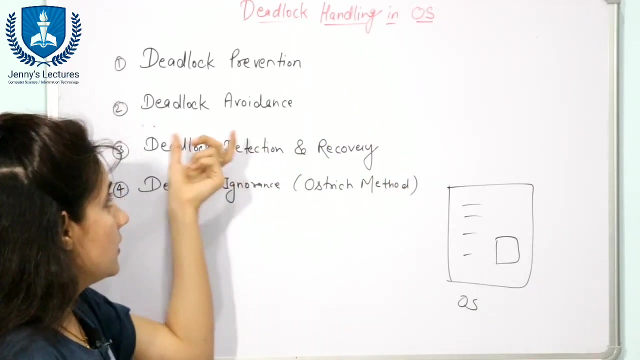 deadlock in this case, then obviously you are adding one more functionality to operating system. then you can say that performance it affects the performance of the operating system also. so we cannot say that always deadlock prevention method would be best. sometimes deadlock ignorance. ignorance is also good, see. next method is deadlock avoidance. avoid the deadlock. this 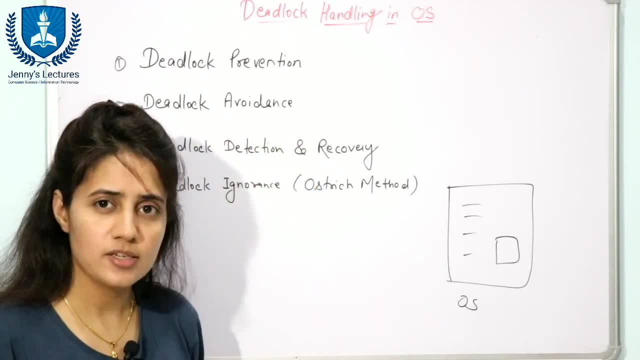 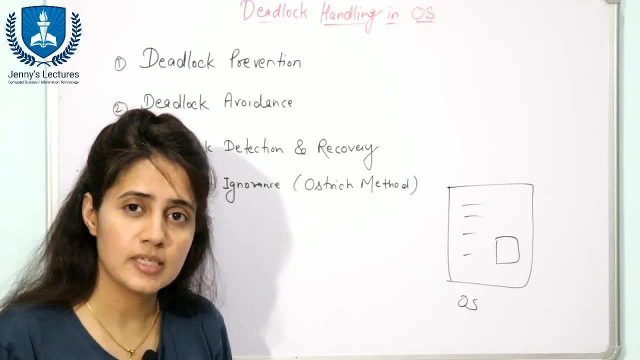 is something kind of futuristic approach. in this case, we, we the system- maintains a table in which it that a process will need how many resources to complete its execution, fine. and when any process request some resources, then the system checks that if that request has been fulfilled with the value, with the resources which are. 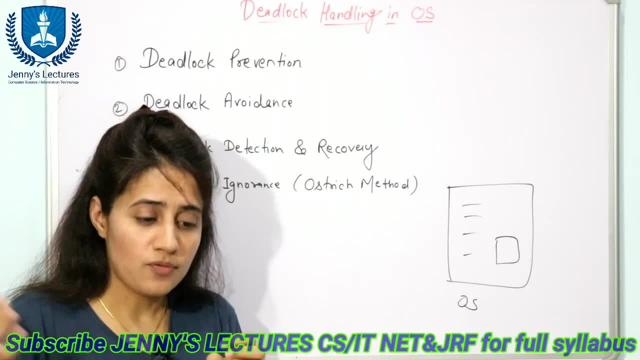 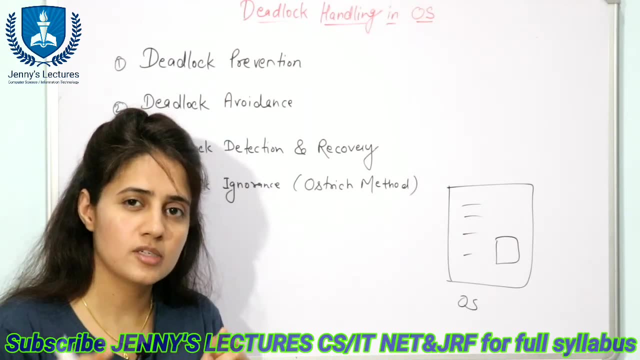 available, then if the system goes after fulfilling the, after fulfilling though that request, if that system goes to unsafe state, then the operating system will not fulfill that request. and if, after fulfilling the request of that process, the system is still in safe state, then the process, then the that. 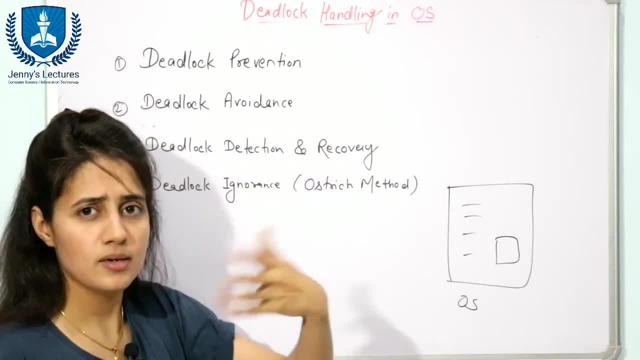 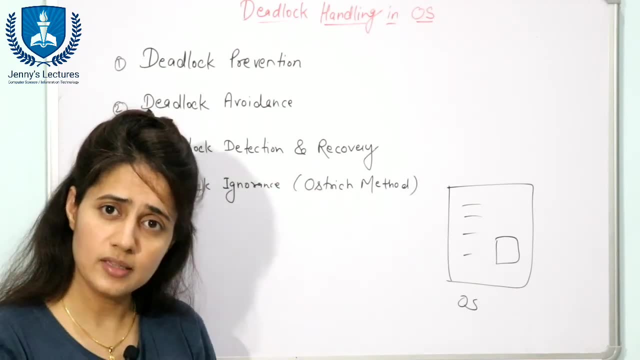 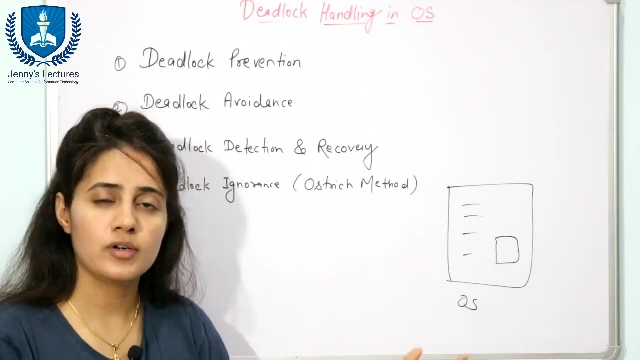 operating system will fulfill that request. we will discuss this case in next videos in detail. fine, now what is deadlock? detection and recovery? as the name suggests, let the deadlock be occur. once a deadlock occur, detect it and try to resolve it. try to recover from it using some methods, though those methods. 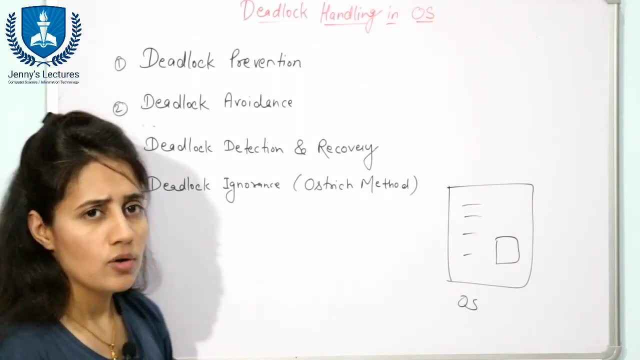 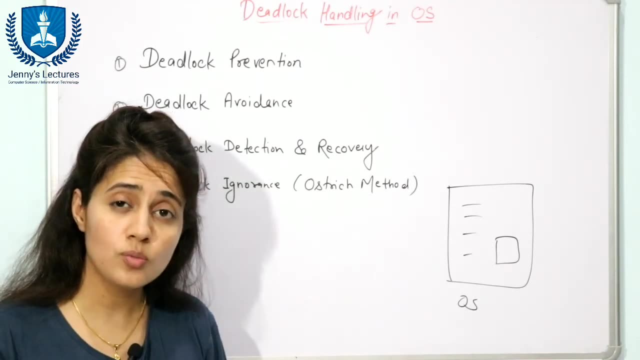 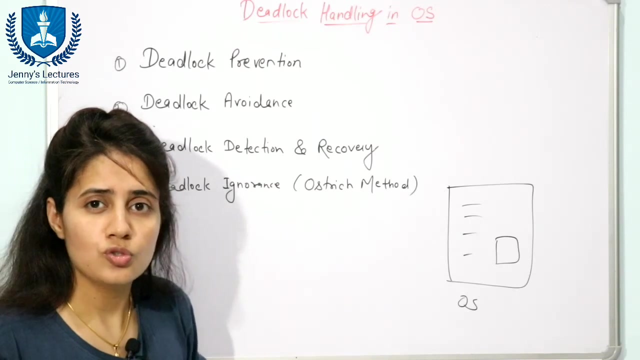 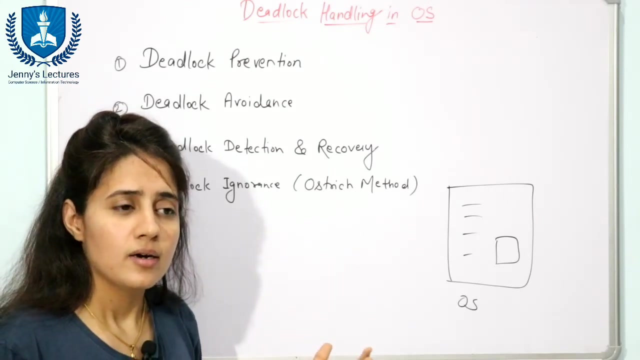 we will discuss in next video. last one is deadlock execution, or you can say ostrich method: simply ignore deadlock. it is assumed that deadlock will never occur in the system. so this kind of technique is used in your Windows and Linux operating systems. why so? because they think that deadlock 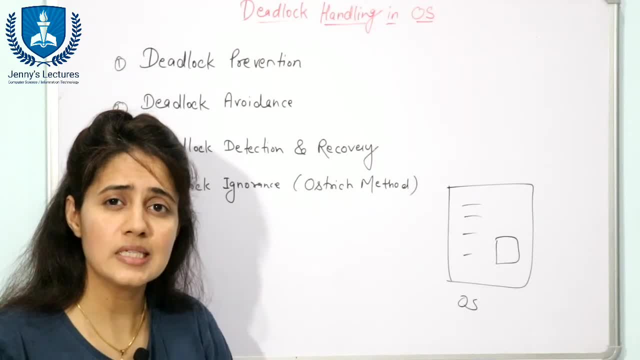 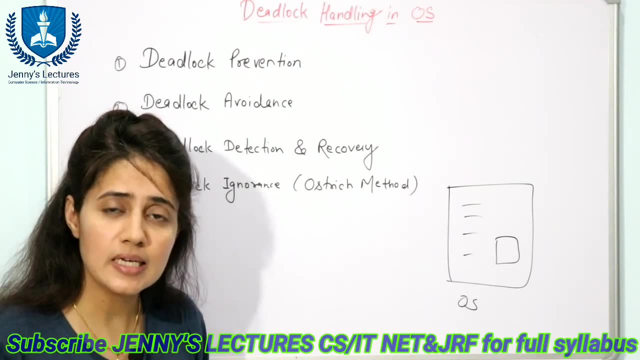 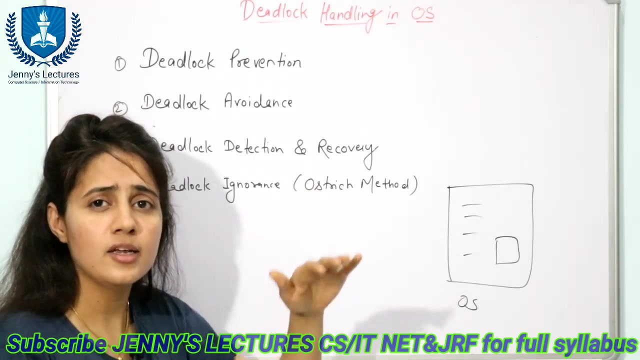 occurs very rarely, once in a year. and if you write so, why why then? if dead lock occurs once in a year, very rarely, then what is the use to write a full fleshed code, a complete code for handling the deadlock, which requires so much efforts to write? it is very complicated code, obviously, handling a 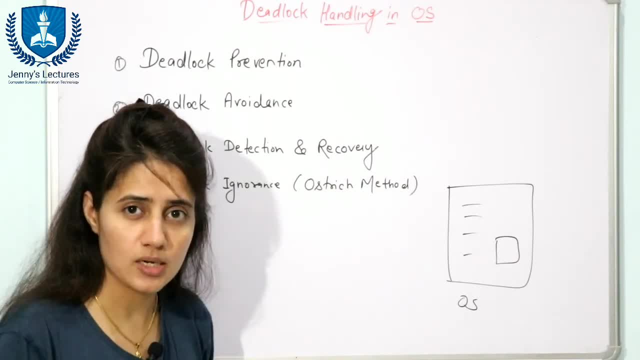 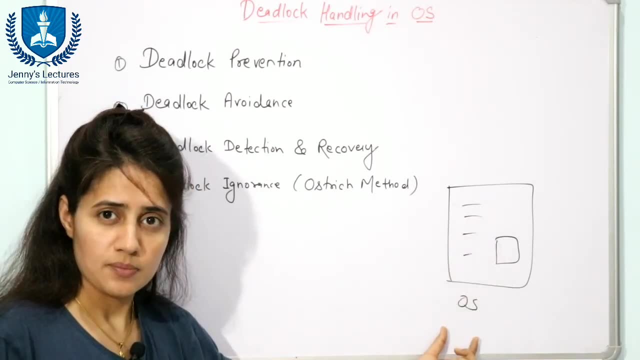 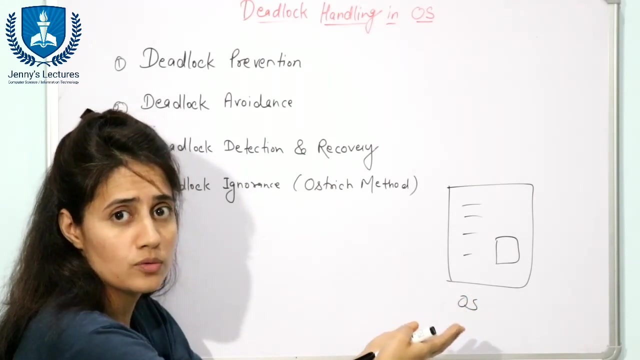 deadlock. preventing a deadlock is not very easy task, so writing this code is very tough, fine, and it also affect the performance of the operating system. as I have discussed, operating system is having some functionalities and one more functionality you are adding that you have to handle the deadlock also. 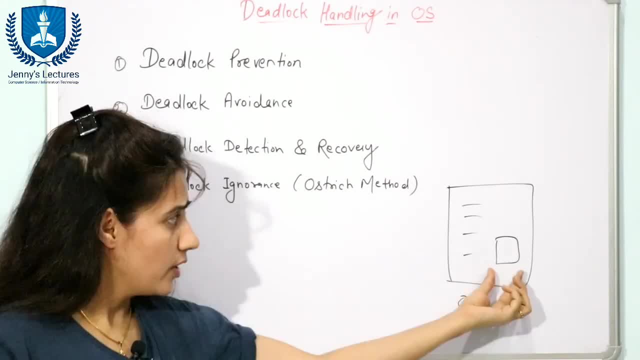 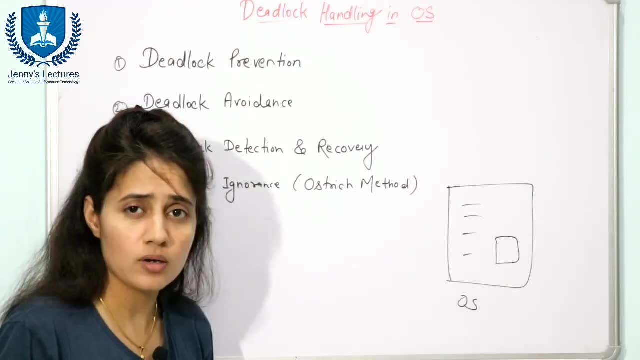 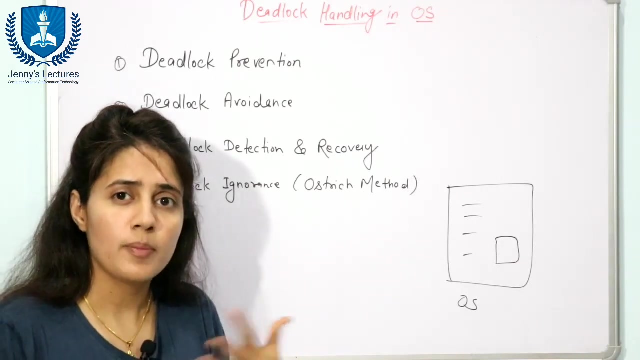 there. obviously performance will be affected of operating system and why you are adding extra button to operating system when deadlock occur- very rarely once in a year. and if deadlock occur then you can easily reboot that system. see, this kind of technique, deadlock ignorance kind of technique- is used in operating system. 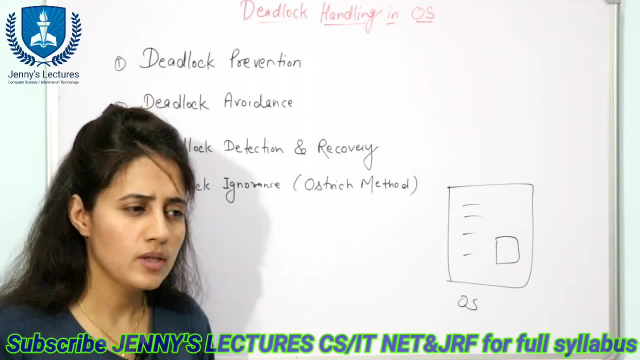 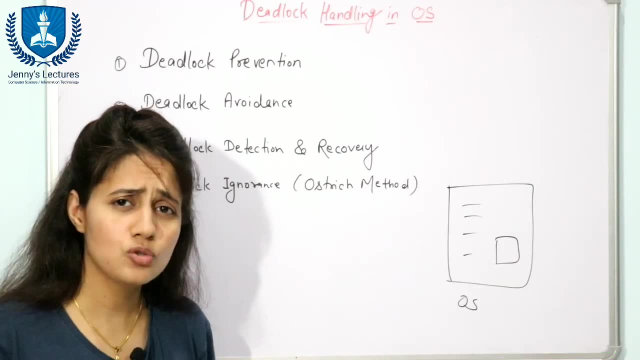 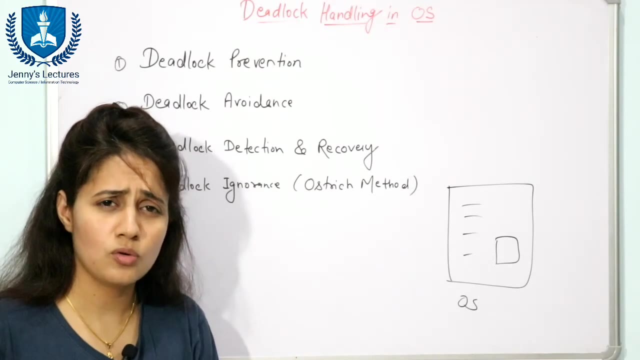 which are basically, you know, used by end users. end user meaning we, the end users, usually use our laptop for may be browsing or some normal stuff. so it's very, you know, common for us to reboot our system. may be when system got hold, we just power of the system, we shut down the system and restart it. 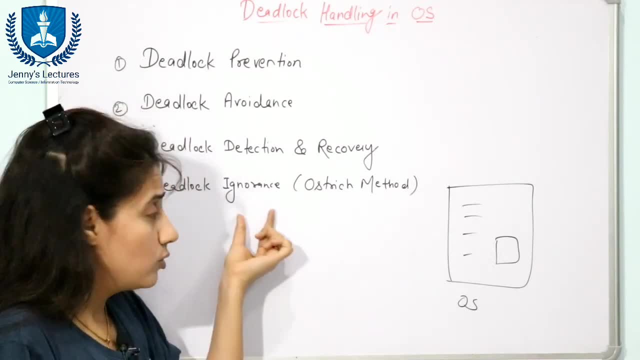 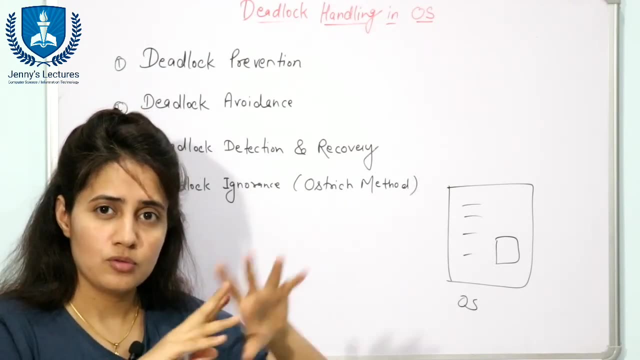 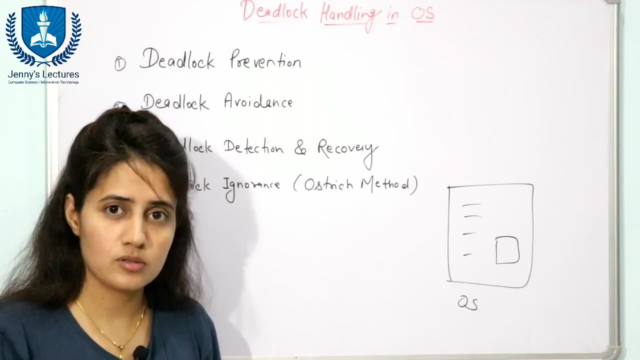 and that is very common for us. but see, deadlock, ignorance is not applicable in some kind of situations like in a aircraft, or you can say in a in a, in a aeroplane maybe. obviously there are some systems, operating system is also there and which is handled by pilots and all something like that. 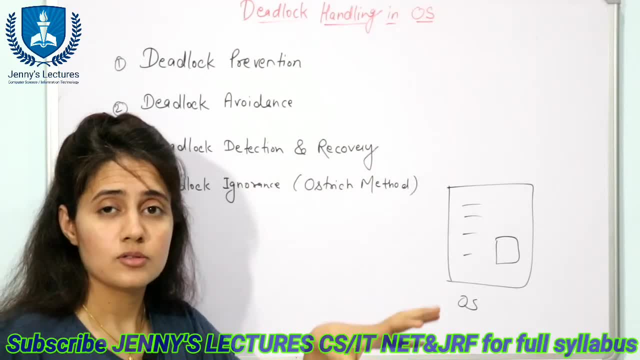 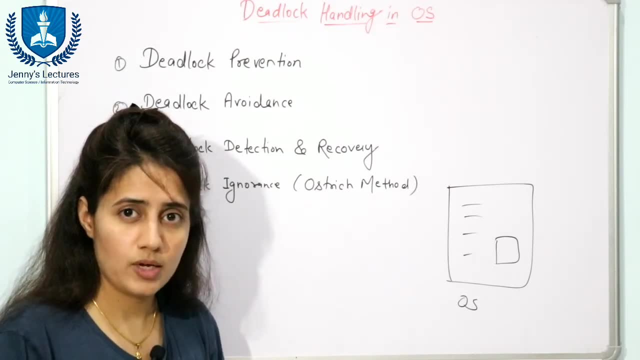 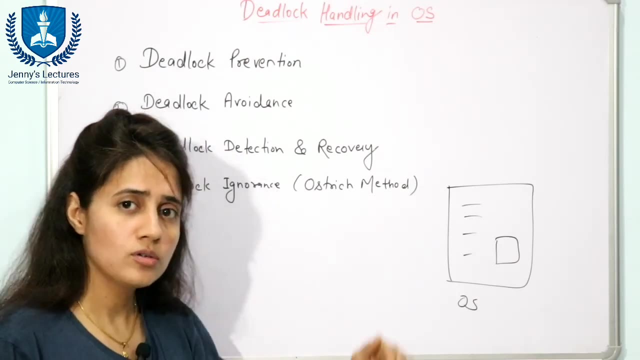 and suppose in the middle of the flight deadlock occurs. in that case what happens if system is not working, you are not, the pilots are not able to control the aeroplane, then what will happen? it is very risky, fine. so in that kind of system we cannot say that deadlock ignorance is a good idea. 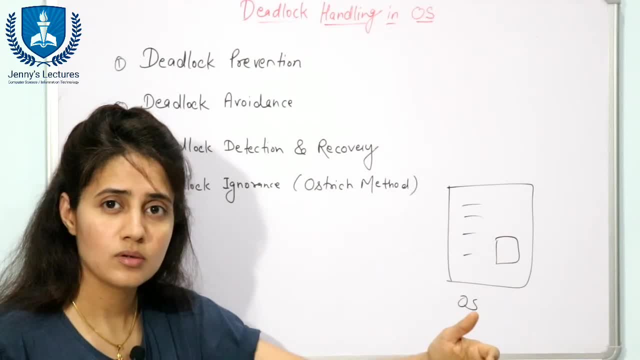 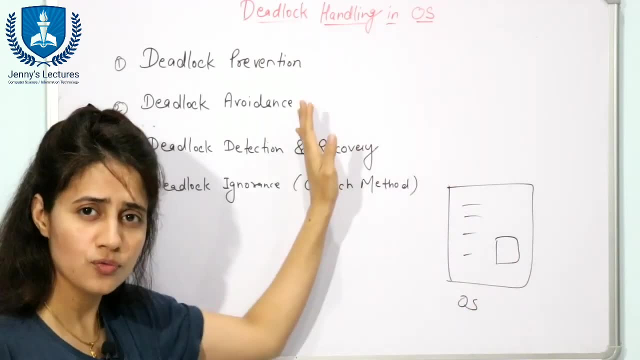 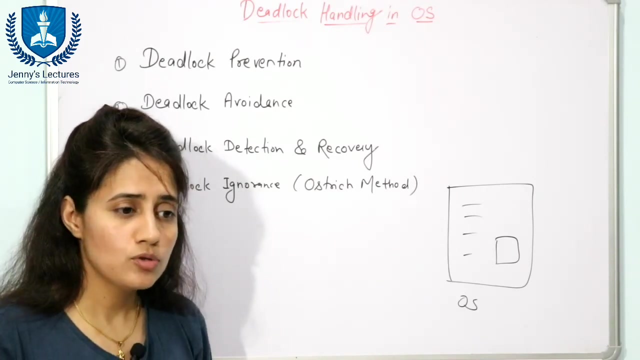 we have to prevent deadlock. although it is, it is, it requires lots of effort and all, but you have to handle the deadlock. so which, which method will be applied when it depends on the nature of the problem? second thing is, if suppose in you can say you can take example of hospital, many machines. 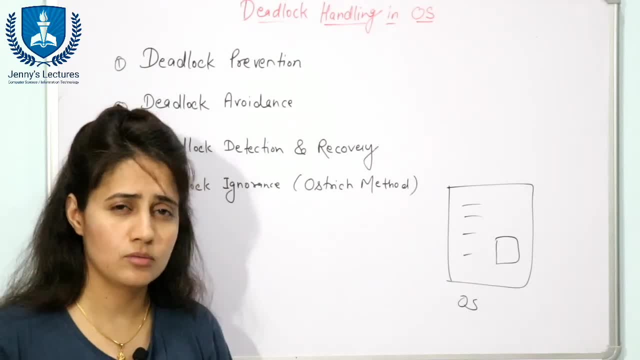 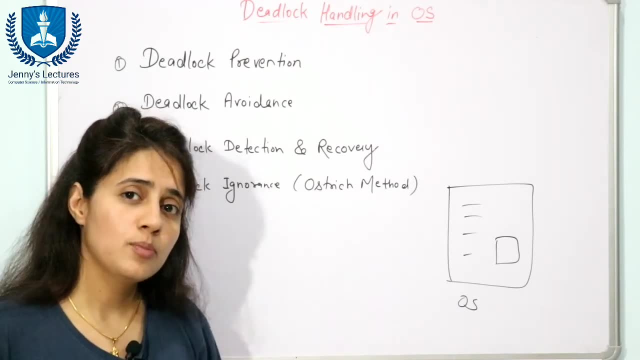 are there today's in, you know, hospital, many machines are there and they are to be operated with the help of, obviously, computers and in there we have operating system also. and in that case, if we suppose that we we follow the rule of deadlock ignorance, then what will happen? 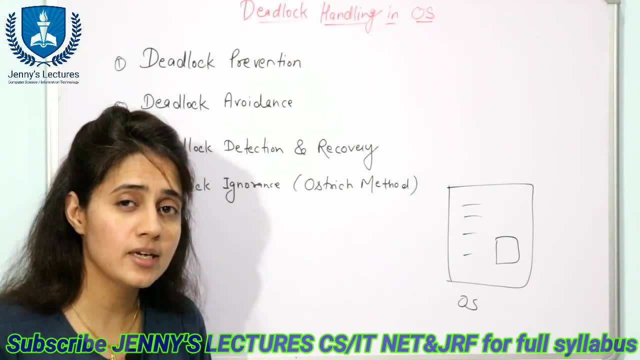 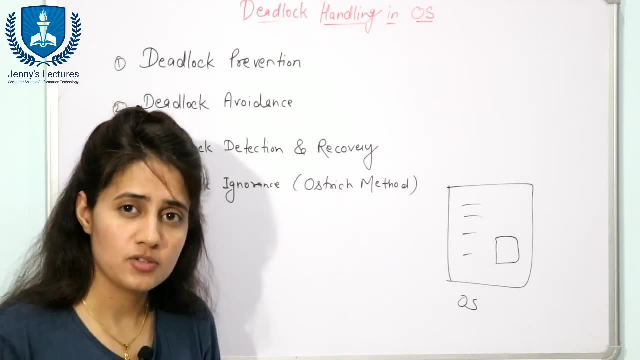 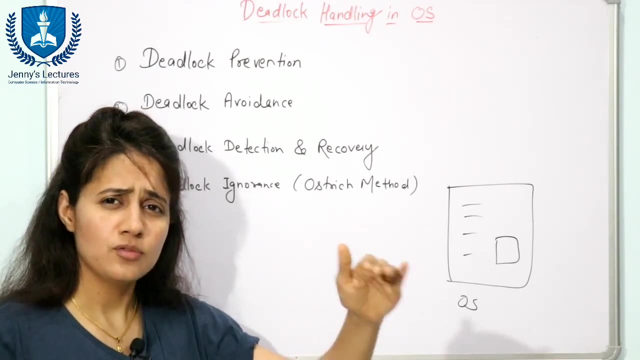 although deadlock appears once in a year, but for once in a year, for that time it is very risky. it can. it can take lives of many patients if that machine is not working. working maybe it is possible. so in those kind of system when very critical jobs are there, in that case we need to prevent the deadlock. 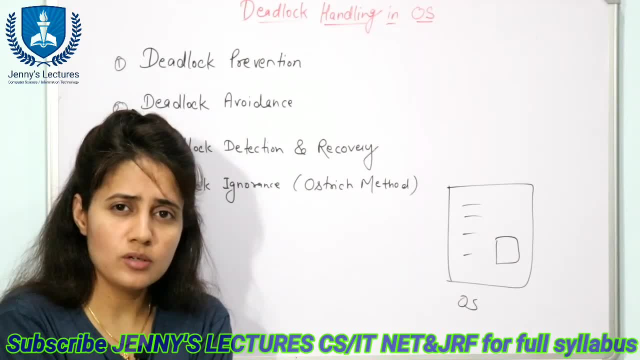 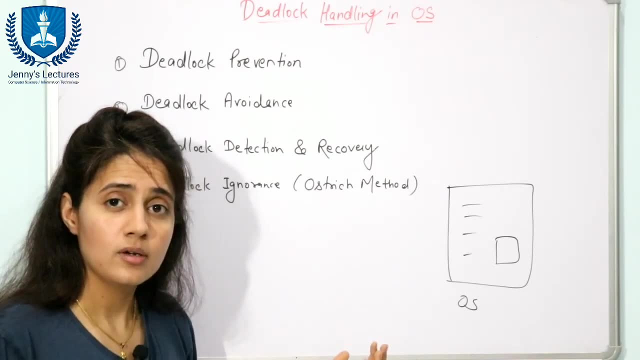 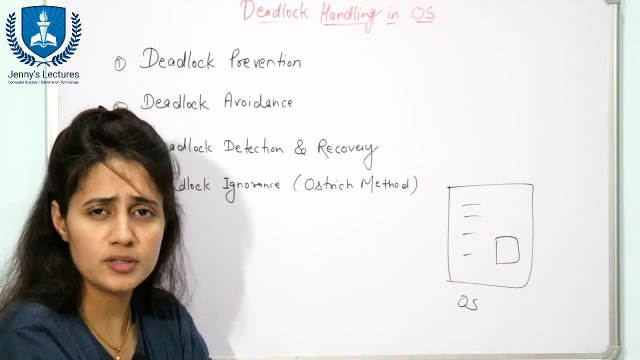 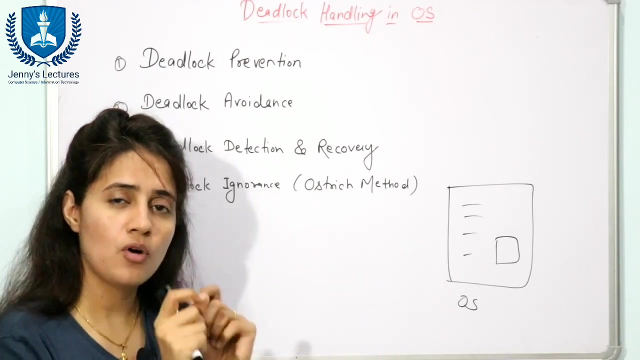 if simple for end user. if you are using for end user systems, it is better to ignore the deadlock rather than putting so much efforts in developing in writing the code for handling or for for preventing the deadlock. for avoiding the deadlock, this is of no use. fine, because basically end user wants what performance or speed they. they do not focus on correctness. we are not any doing anymore things. 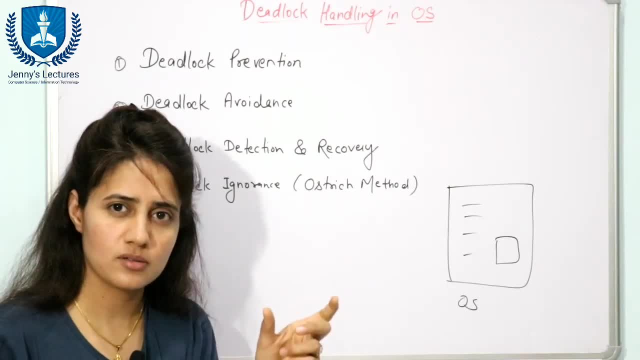 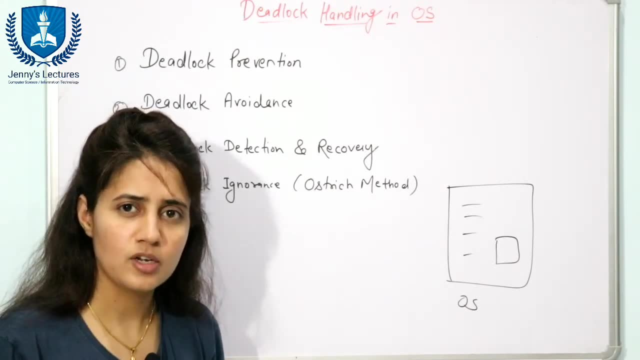 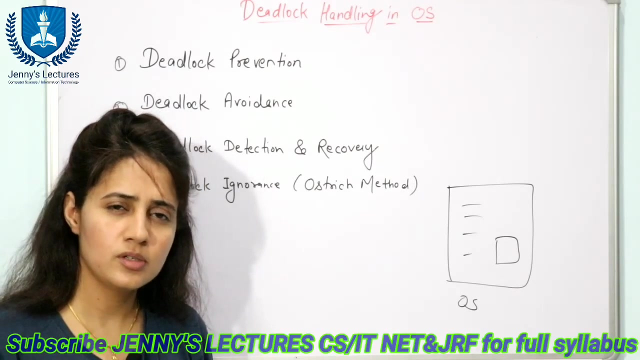 they are focused on the brain and they are not doing anything else, any scientific task or something like missile launching and something like that, fine. so we want speed of performance. so if, for some amount of time, for two or three seconds, our system would hold, then we simply just restart our system and that is fine with us. fine, so these are the four. 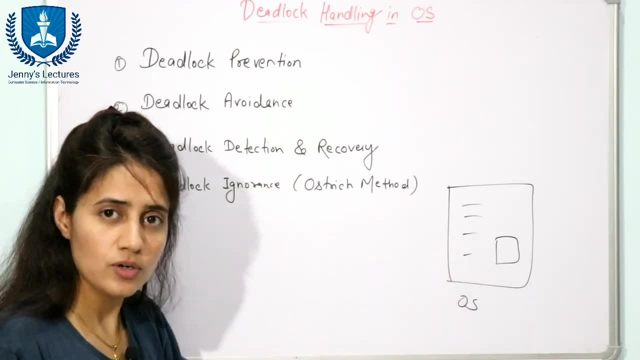 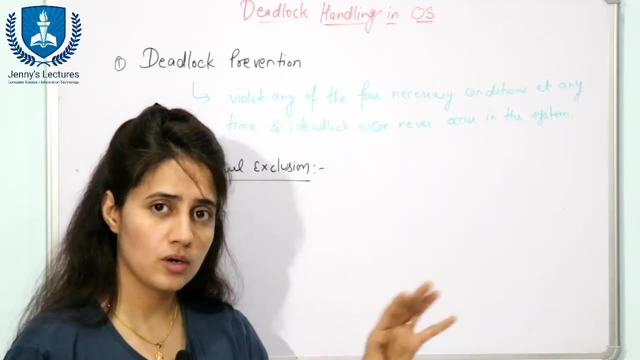 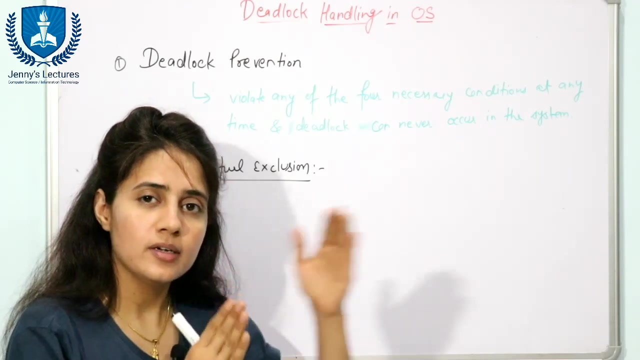 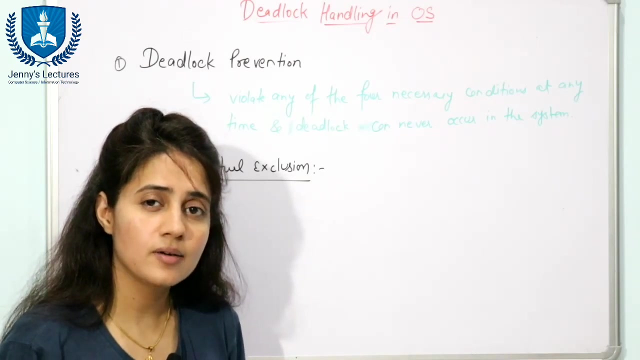 techniques. we will discuss these techniques in details, one by one. in this video i am going to discuss with you deadlock prevention technique. see, we have discussed four necessary conditions for occurring deadlock: mutual exclusion, hold and wait, no preemption and circular wait. now, how to prevent deadlock? if suppose you design a system in such a way that any one, at least one at least, 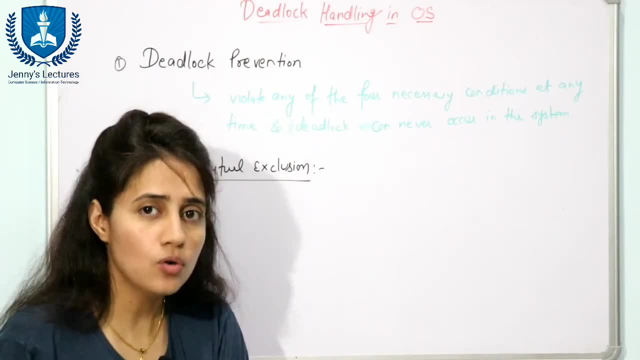 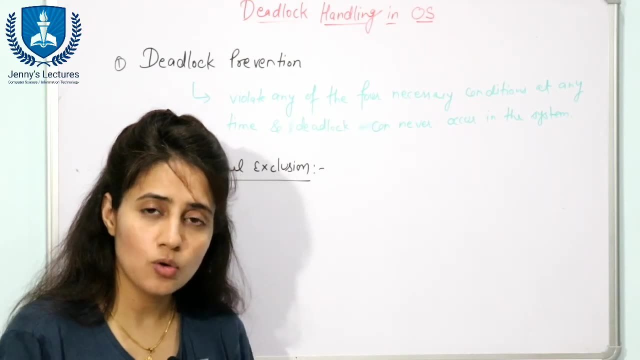 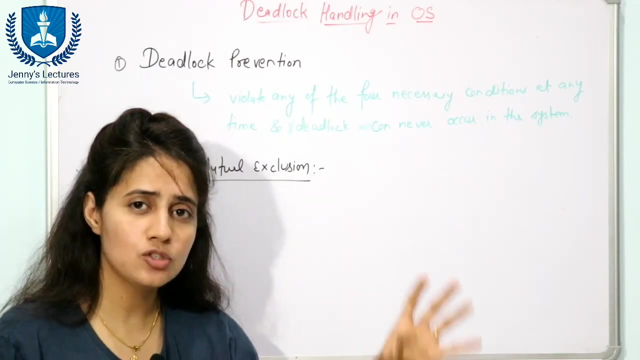 one out of the four conditions cannot hold in the system, then you can say that deadlock will never occur in the system. i am not saying that all the four conditions you have to fail all the four conditions. no, at least one condition. just violate at least one condition. 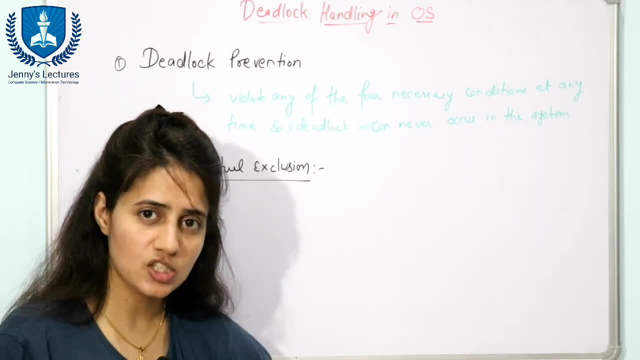 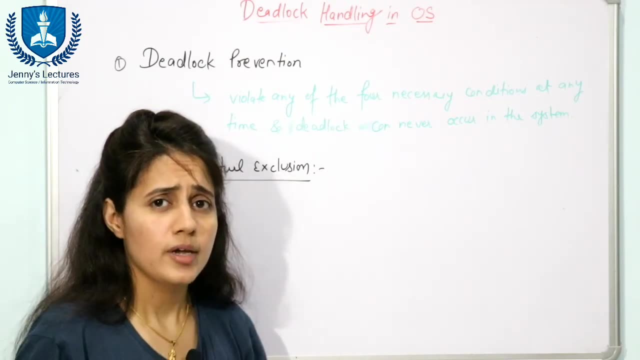 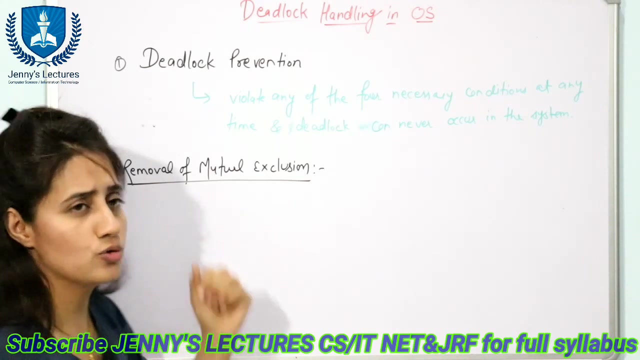 from the four, uh, from the four necessary conditions, and then, at any time in the system, and then deadlock. you can say that deadlock will never occur in the system. so first condition was mutual exclusion. so you can say that first is first point is removal of mutual exclusion. you, 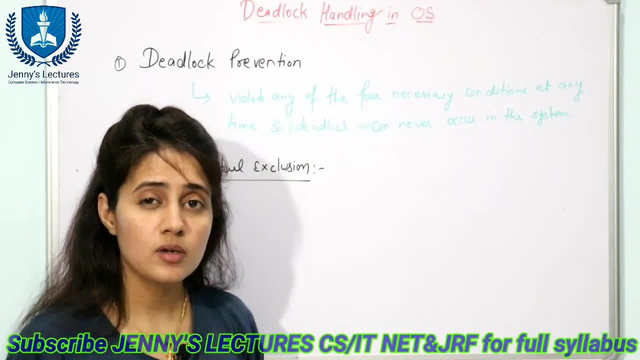 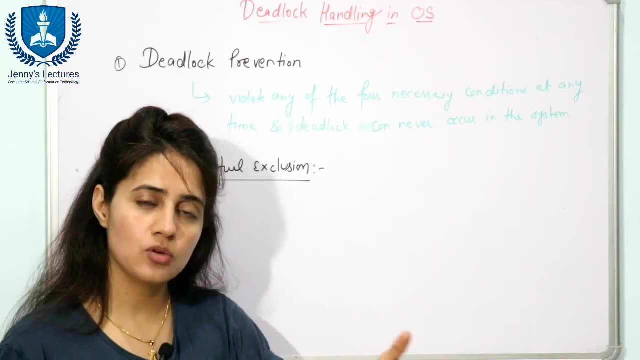 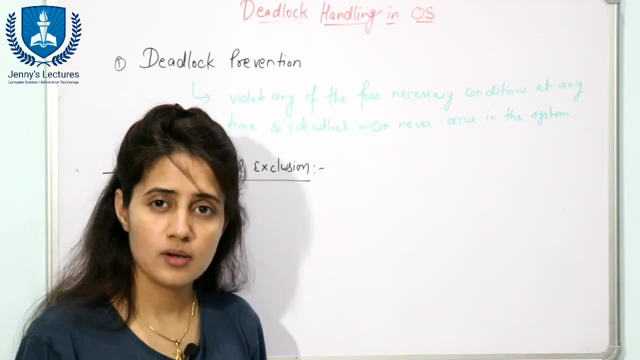 have to remove mutual exclusion. now what is mutual exclusion? at least one resource in the system should be known. shareable means only one process can use that particular resource at one time. now how to remove mutual exclusion? make all the resources shareable. but that is not so easy and almost impossible. this is in implementable. we cannot implement this. 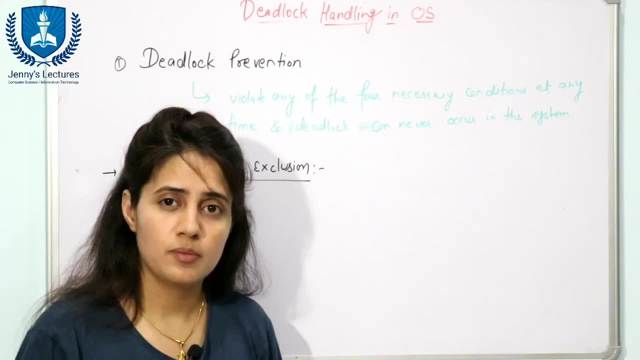 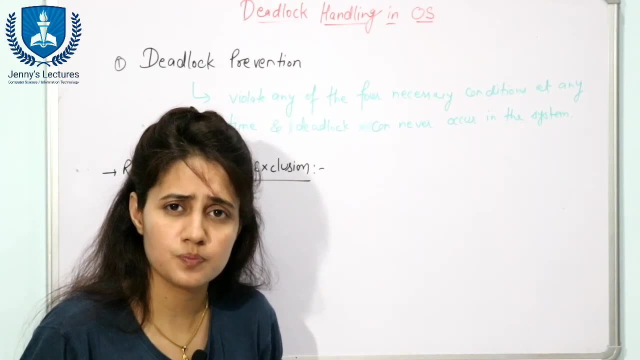 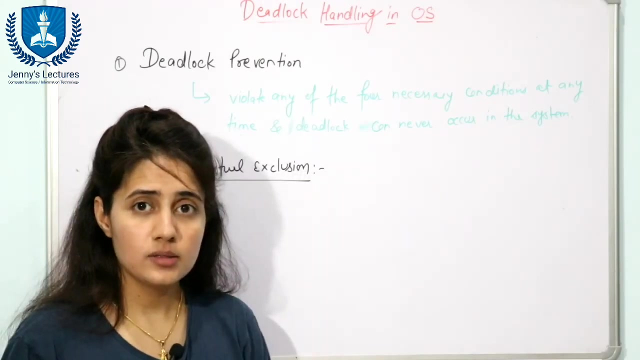 and this method. we cannot make all the resources shareable because some resources are inherently non-shareable. you cannot make those resources shareable, like a printer, that is non-shareable resource, although in case of printer, the spooling method can be used. now, what is this spooling method? see the memory which is associated with. 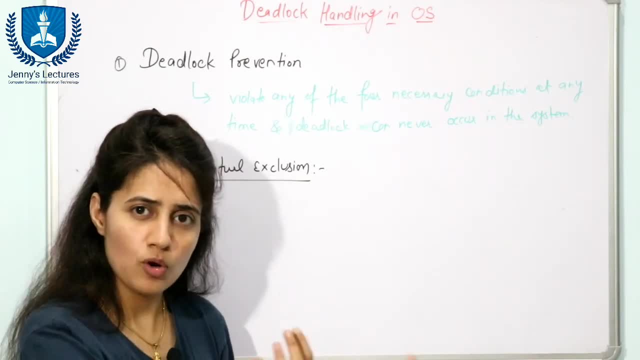 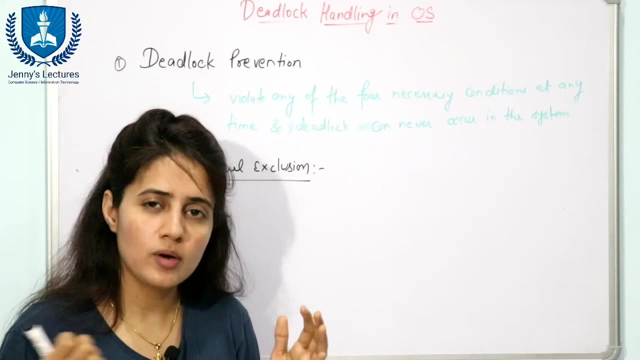 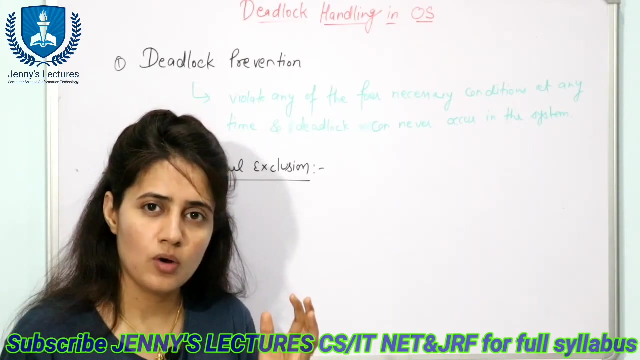 that printer takes jobs from all the processes, fine, and after that printer will collect all the jobs and print one by one in first come first, sir. so process need not to wait for the printer. process can do its own work. that is spooling, basically, but this pooling is also a technique. 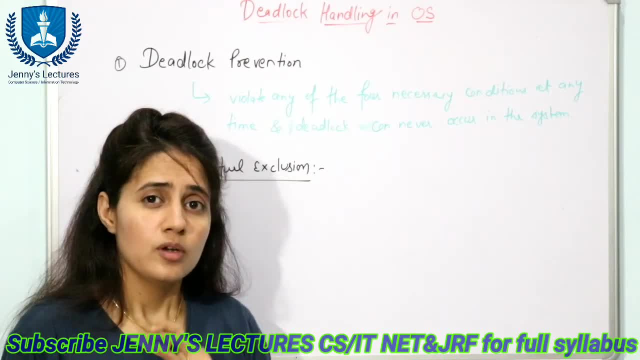 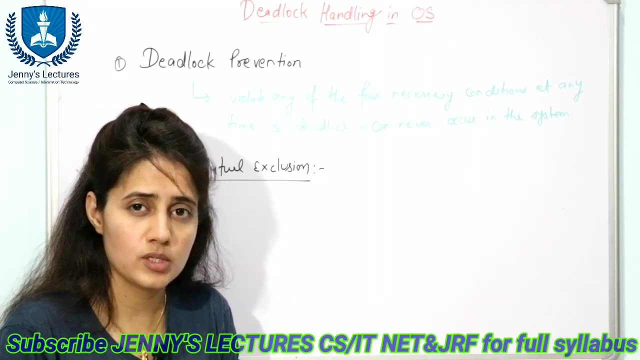 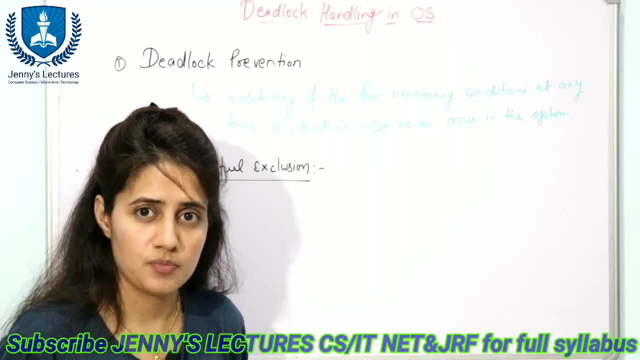 which cannot be applied to every resource. so we cannot make some resources shareable, and if you force a resource to be used by more than one process at one time, then maybe some very serious kind of problem may arise in the performance of the system. so this is basically infeasible. 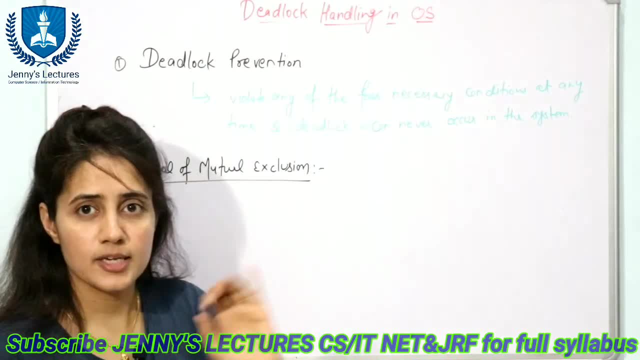 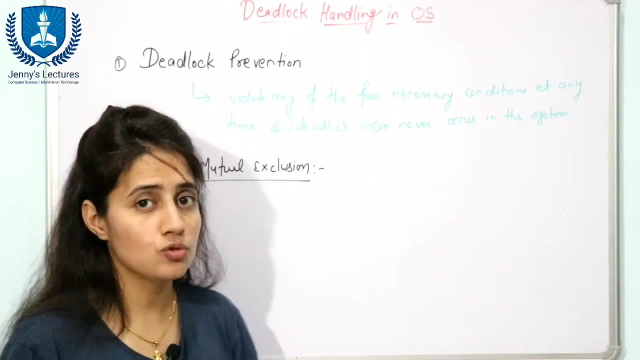 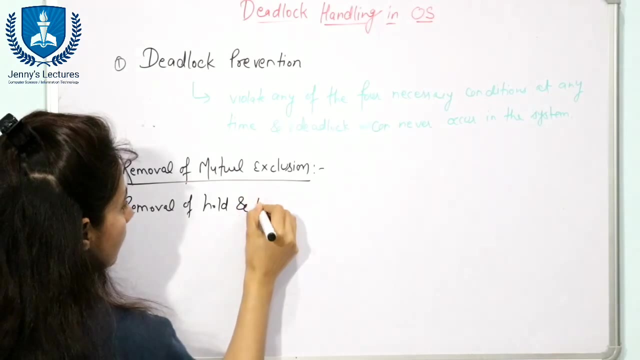 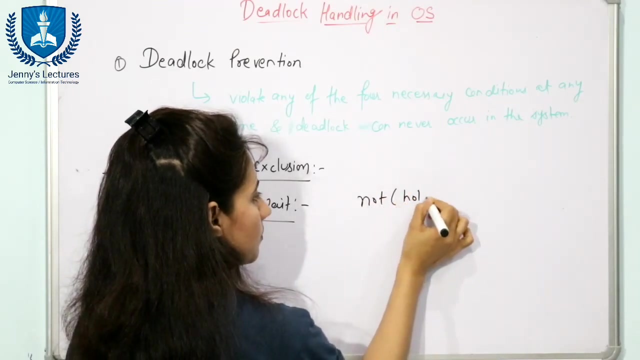 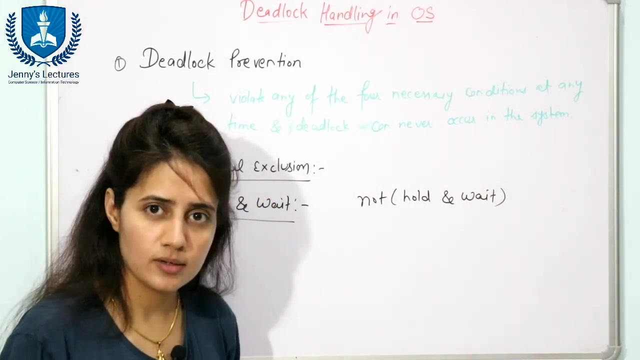 not feasible to implement the removal of mutual exclusion. fine. second technique is was hold and wait, so you have to fail that condition. so you can say that second point is removal of hold and wait. or you can say not hold and wait, negation of hold and wait. or you can say either hold or wait. now how to remove this technique? how? 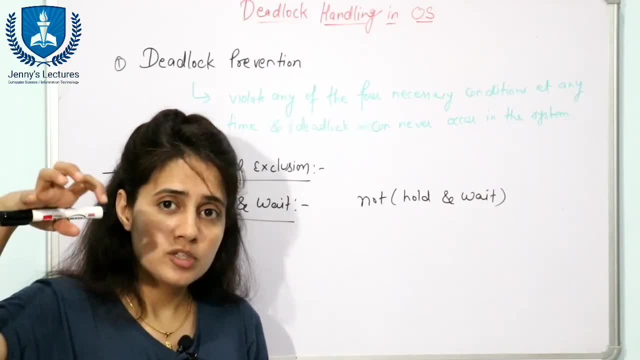 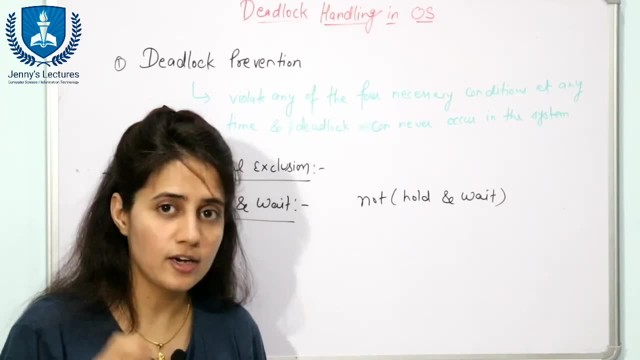 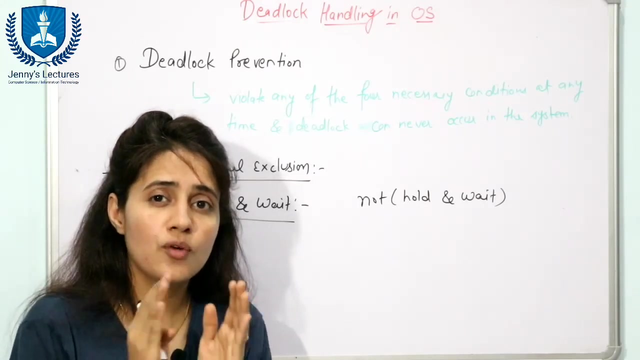 to fail this hold and wait technique. what is hold and wait first of all process is holding some resources and requesting for another resources. or you can say, waiting for some another resources. fine, that is hold and wait. but you have to remove this hold and wait. so you have to make sure that when a process is requesting for some resource, 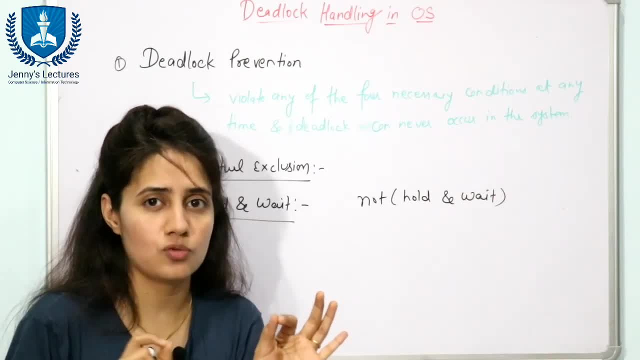 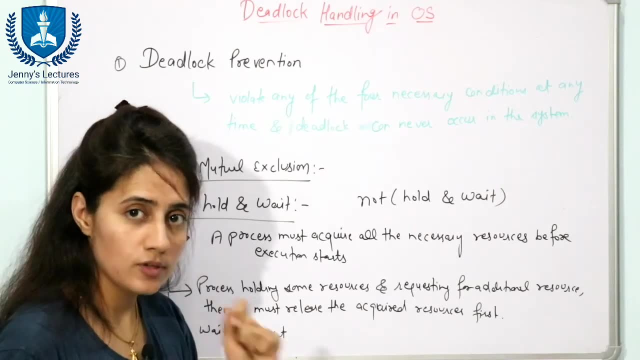 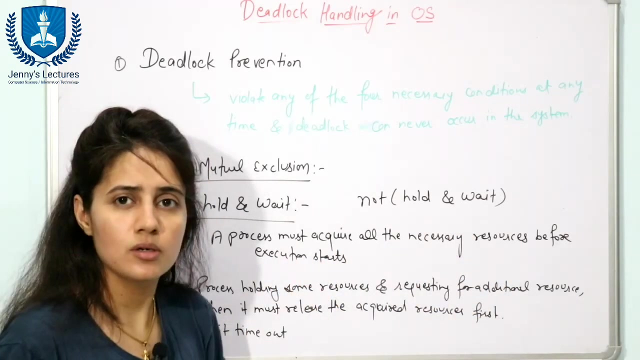 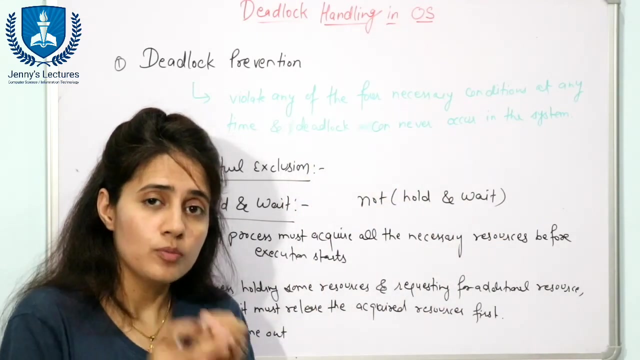 then that process is not holding any resource. now how to you can, how to ensure this thing? there are three methods. first is first is see a process must acquire all the necessary resources before execution starts. suppose a process wants 10 resources, fine, so before its execution starts. 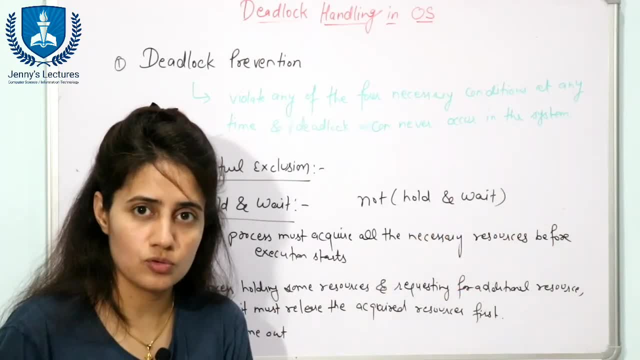 the process must acquire, must hold all the 10 resources. after that it can start its execution. let us take one, one process. let i want to you know, print some document, and first of all i i'll make the document in ms office. so i need my laptop and i want to print that also. so two resources. i. 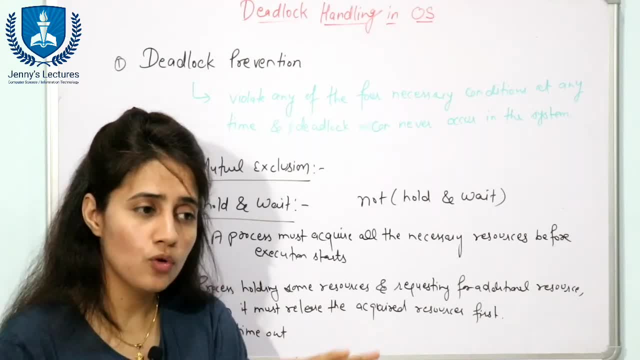 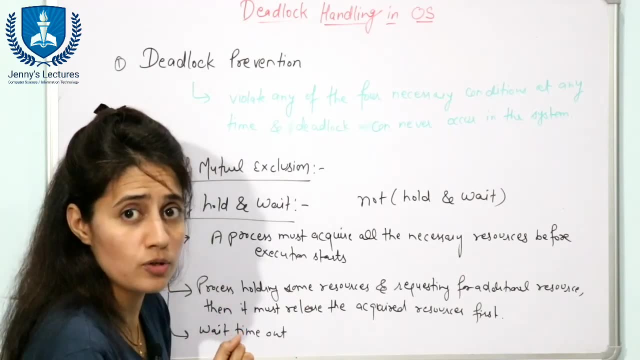 need. one is laptop and one is printer. so before i start typing the document i acquire printer also. so we have laptop plus printer also. now suppose when i am typing that document i need maybe 10 minutes, 15 minutes, half an hour or one hour. till then the print, i have acquired that printer. so 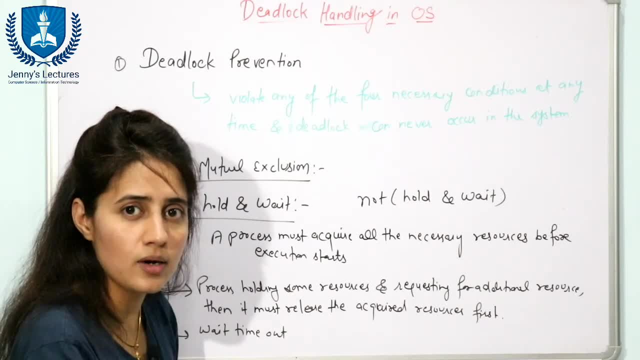 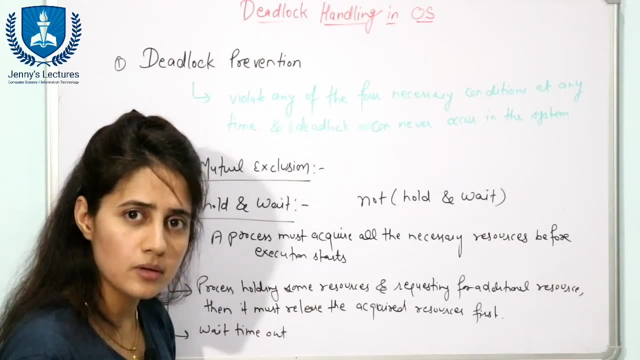 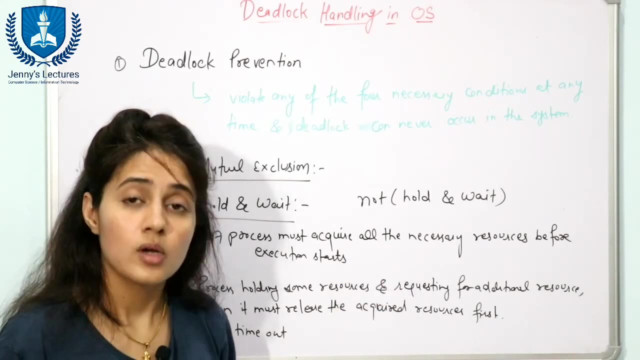 this is what that is: wastage of that document, that printer, while I, while I am working on my own MS word. till then any other process can use that printer and after that I can use that printer. so the drawback of this approach is resource utilization would be very low. second thing is this kind of approach is practically 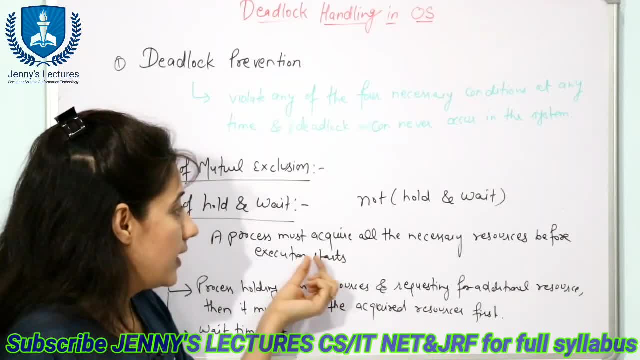 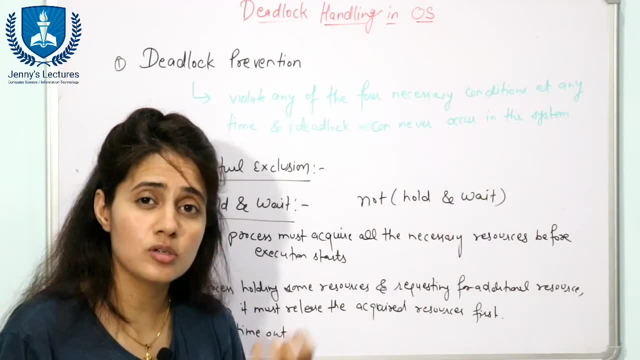 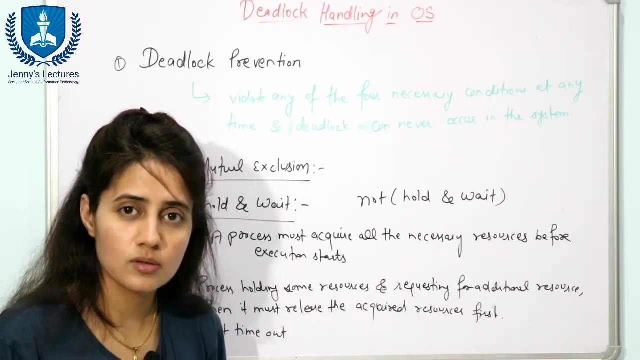 not feasible to implement. why so? because, at starting, only process need to acquire all the resources it needs for its execution, but it is almost impossible to know how many resources that process will need for its execution, for completing its execution. so that is practically not possible. so see, this approach is not implementable, practically not feasible. now, 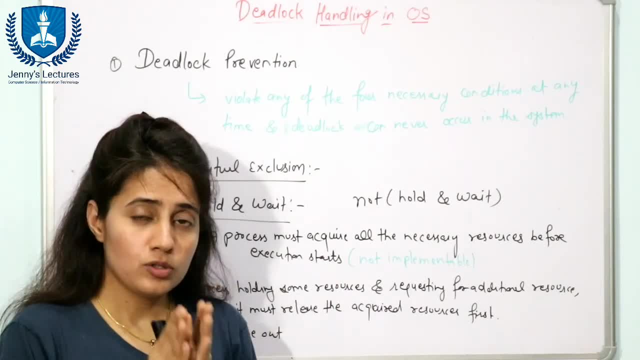 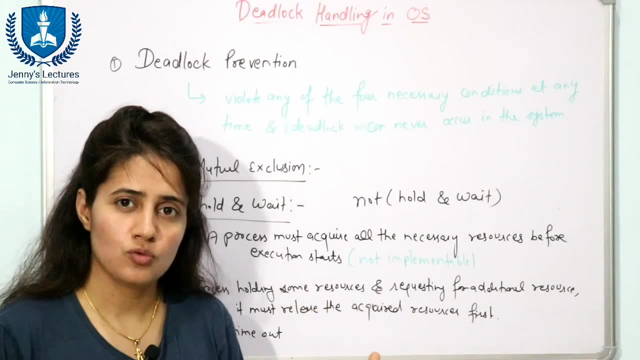 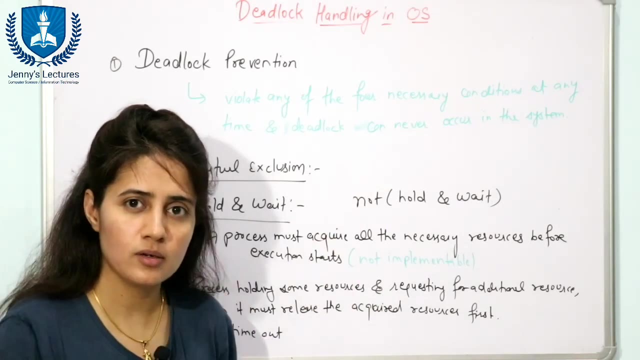 second thing is. second approach is so: see, a process is having nothing at one particular amount of time, fine. now suppose at some point of time it needs only one resource. fine, some, maybe, at some particular point of time it needs only one resource. point of time. I need only laptop. I want to write the document, I don't need. 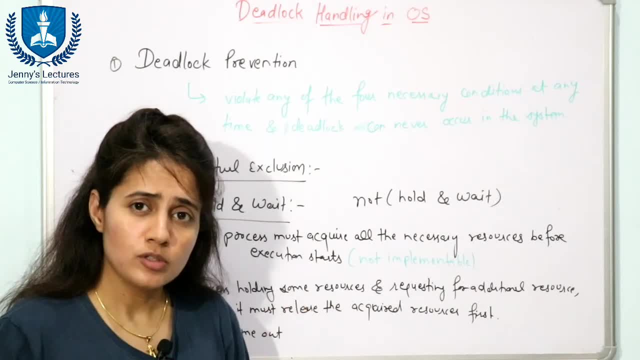 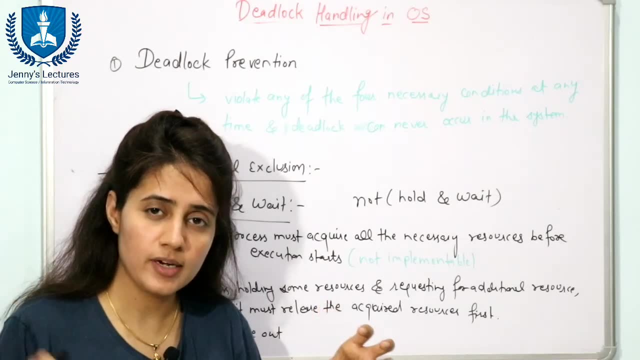 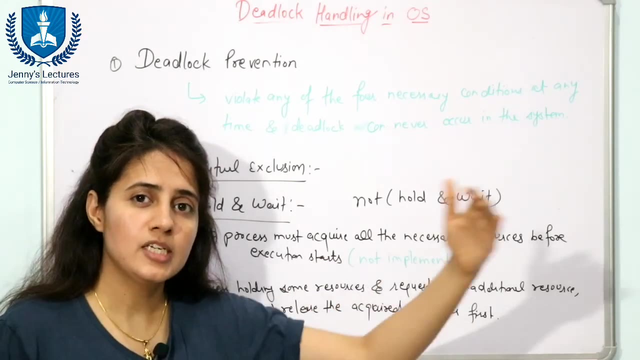 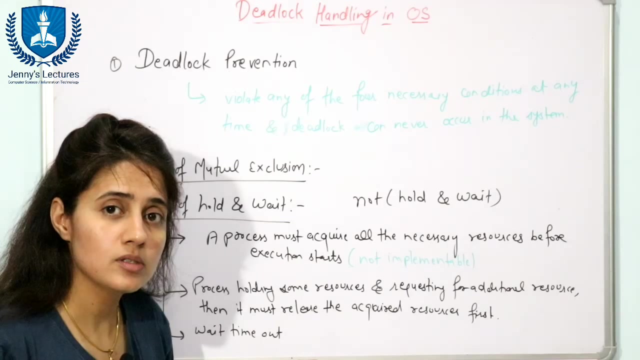 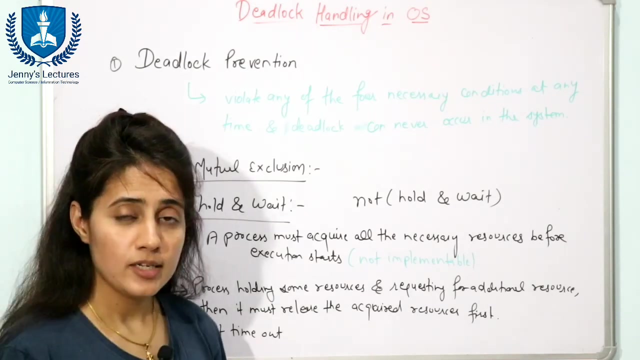 printer. I need printer after some amount of time. so the process will acquire the desired resources. when it has no resource, fine and use those resources. and now, now that process wants additional resource, but before requesting the additional resource, that process has to release all its acquired resources. let us take that example. see, I am writing some document in preparing a. 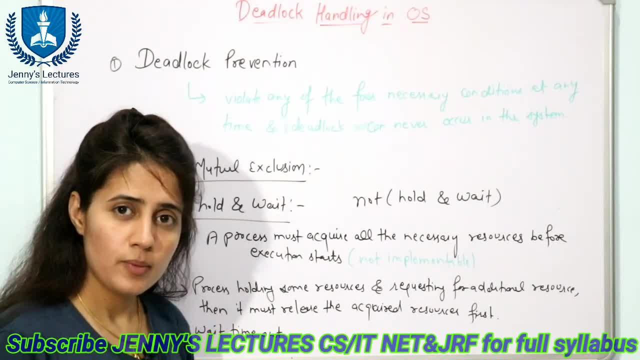 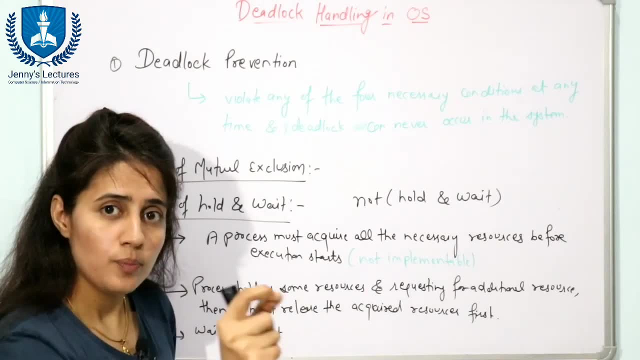 document in MS office on my laptop and I have done with my that that kind of work. now I need printer. but if I request for printer then I have to release laptop. I cannot say that I hold that laptop only. I cannot say that I hold that laptop only. 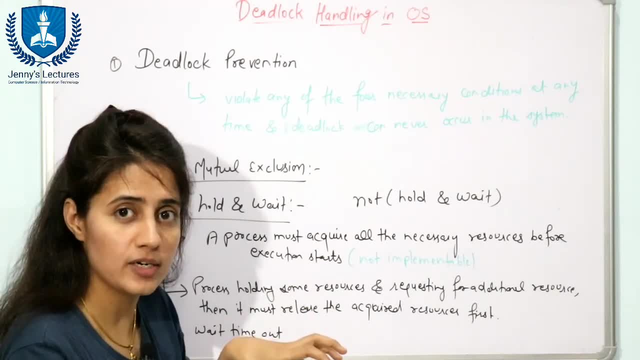 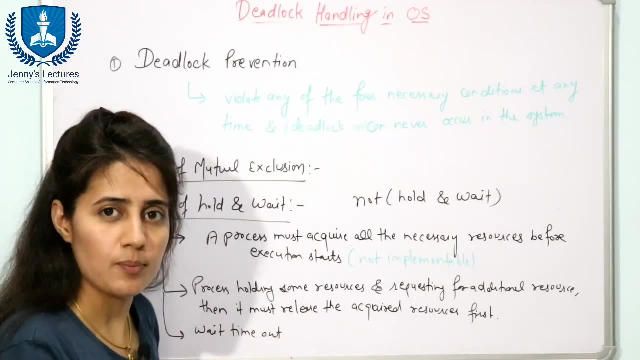 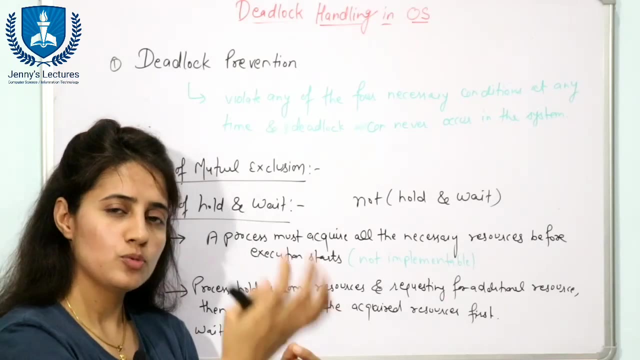 and I request printer also because we have to remove hold and wait condition. so if you are requesting for some additional resource, you have to release the acquired sources. then I have to release laptop, fine, and again in that case after that I can request printer. and if suppose printer is free and I got. 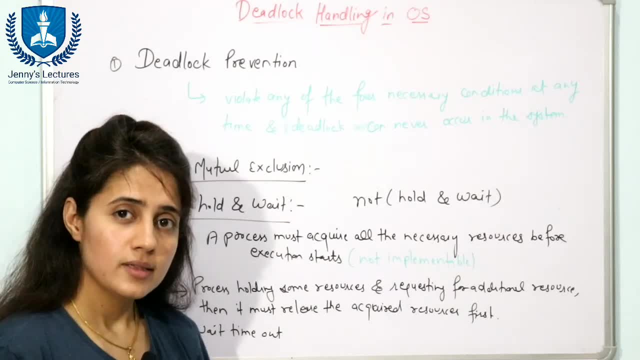 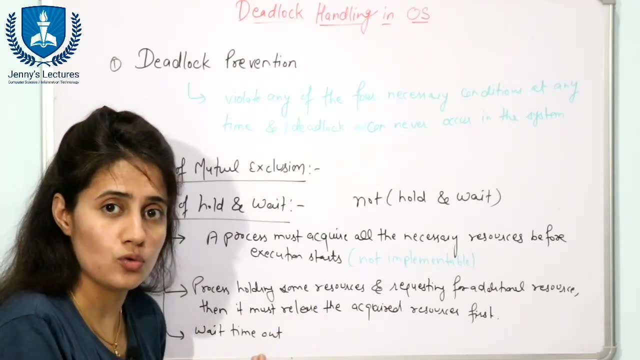 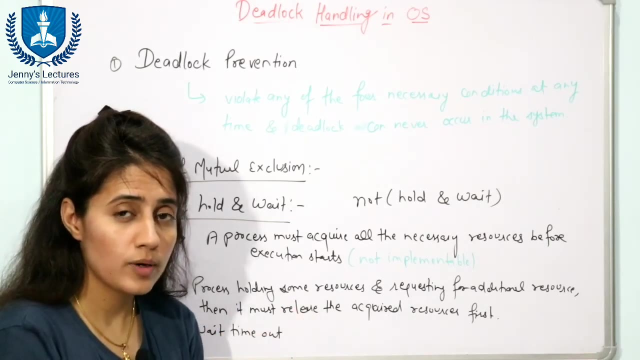 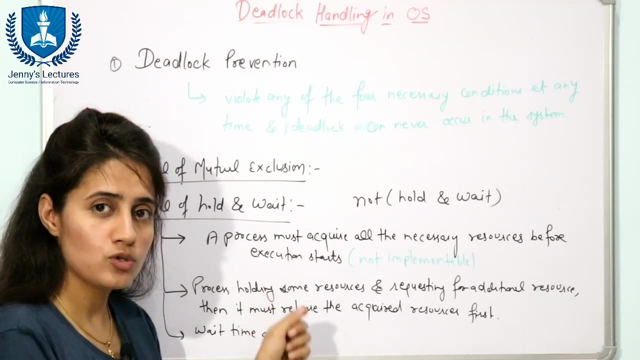 the printer. but in this case what happens? sometimes that process needs that previous, that old resource also, so plus the new resource also, but that process now only have the new resource. but that old, that old resource has been released by the process. now it has to make a request to that old resource. but 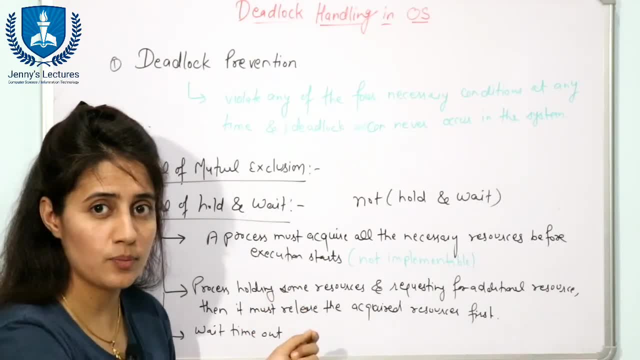 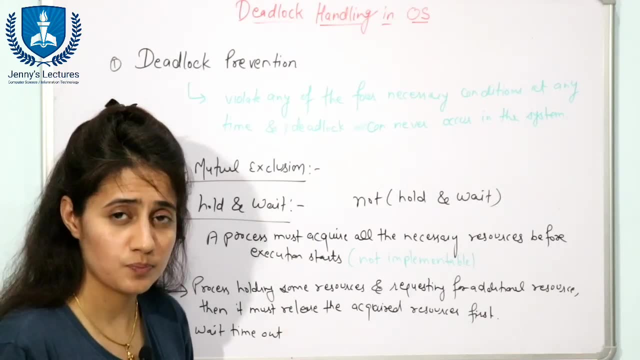 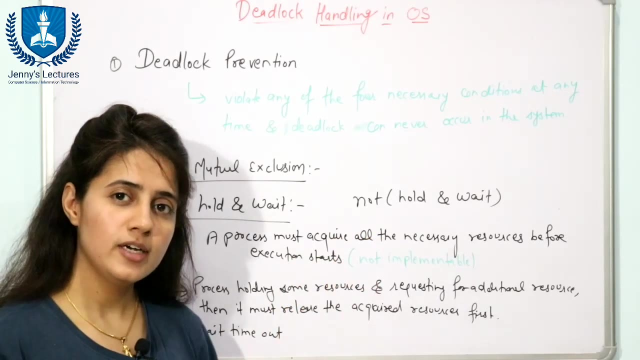 before requesting some additional request, it has to release that printer or it has to release the resource that it have at that particular amount of time. so this thing happens. so see, if I have taken my- you know that word file in my pen drive, then I don't need laptop. I release laptop, I only. 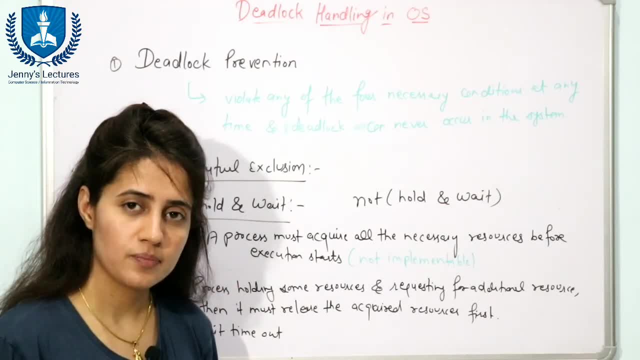 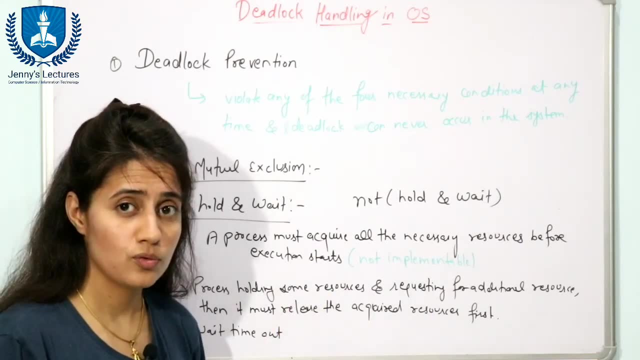 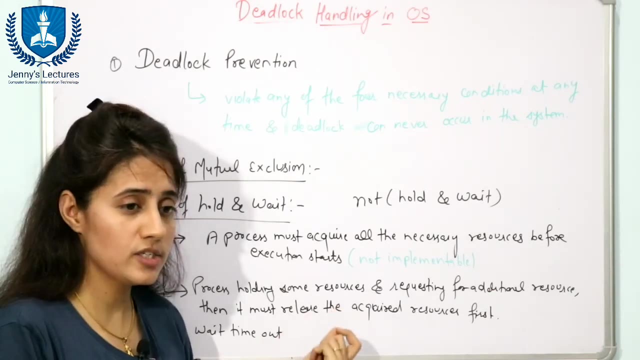 take printer and just take out the printout, so that is fine. but if I didn't take that file into my pen drive, then I need laptop also. fine, but I have now printer. only now I will. I will request laptop, but before requesting any additional resource I have to release printer now. yeah, 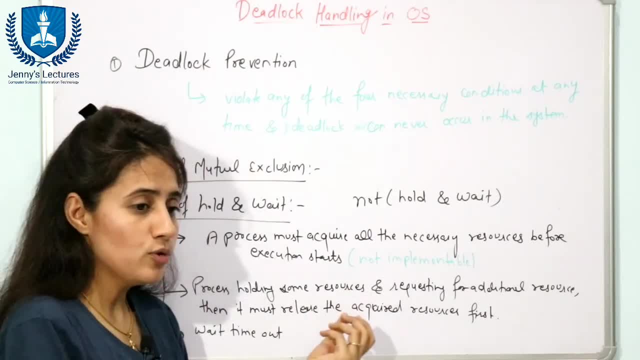 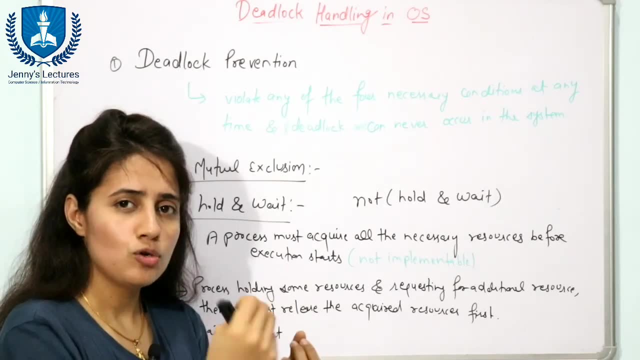 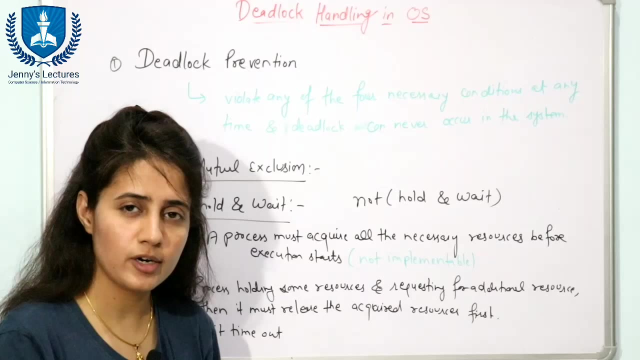 I released printer. okay, now suppose I have a printer, I have a printer, I have a printer, I have. I got laptop. now I need printer. fine, so maybe printer is also free at that particular amount of time and laptop is also free. so I got all the do, all the two resources at the same time. so I 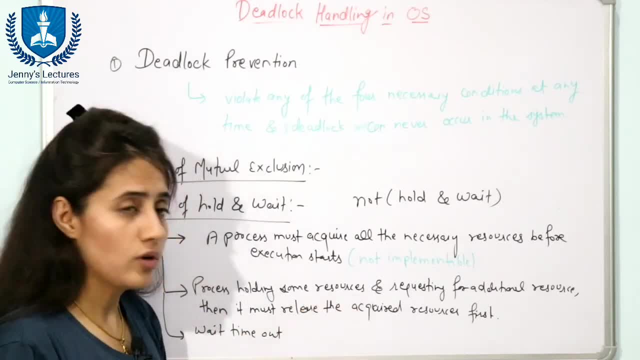 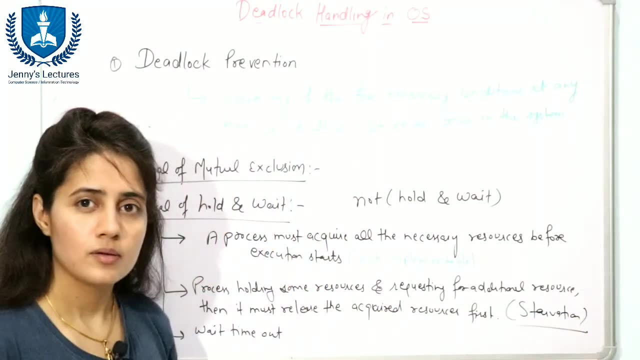 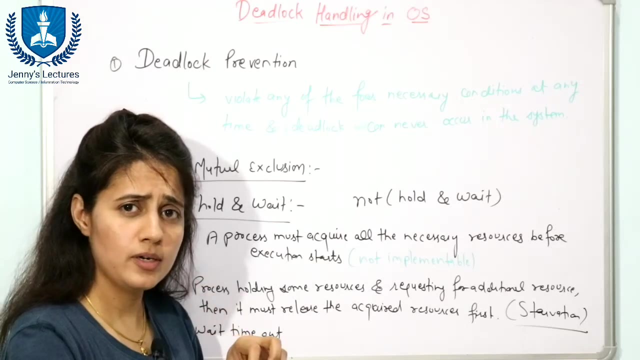 can do my work. but the drawback of this condition is what this, this approach, is? what starvation problem. now, again and again, that thing happens. if I have laptop, then I have to release printer and printer is taken by some other process. fine, now when I request for printer, I have to release laptop. now, if printer I have printer, then I have to make request for. 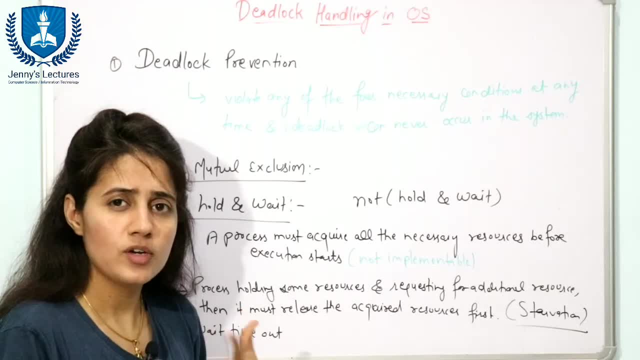 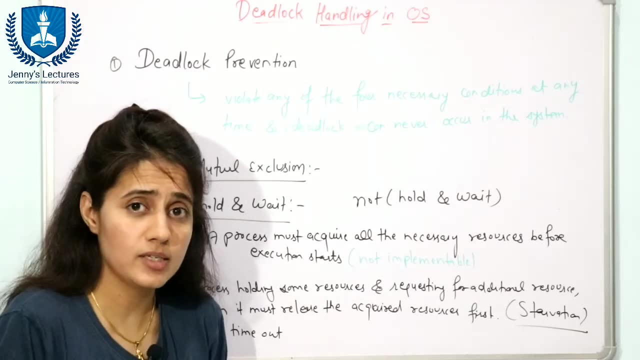 laptop fine. so this, this kind of thing always happens. maybe you have to that one process have to release its resources many times and maybe it is a case that once it is having maybe many number of resources and suppose the process uh is having 10 resources and it needs one more resource now before the any additional request it. 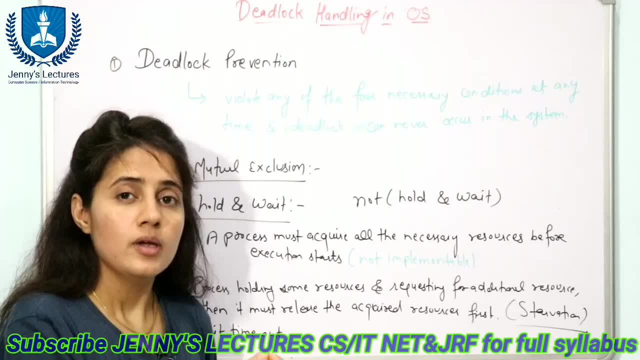 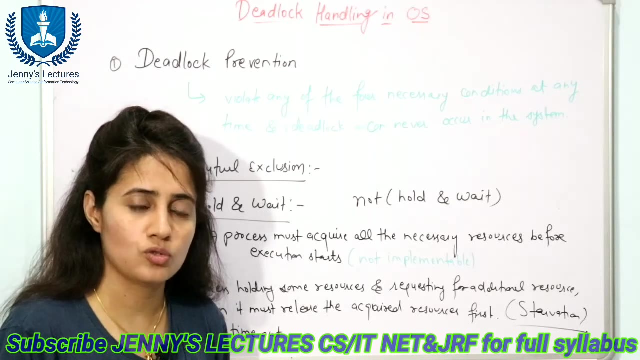 has to release all the 10 resources. yes or no now, maybe after, maybe again if that process request and that process is not able to get so many resources at same time so many times, that process has to release its resources. so starvation problem can be there. so third approach is wait time bound. 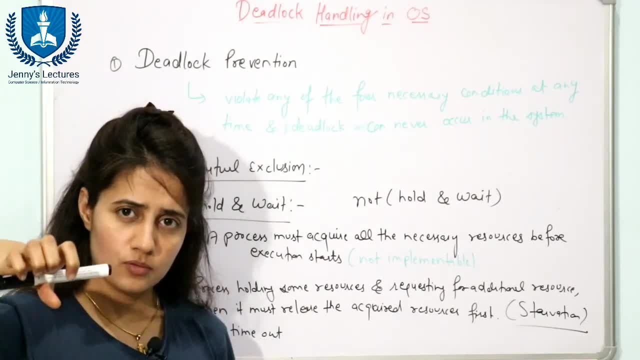 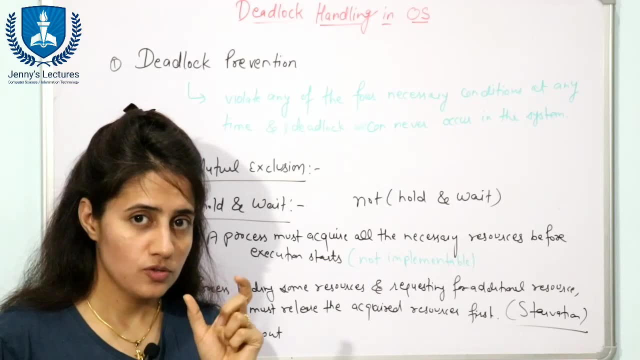 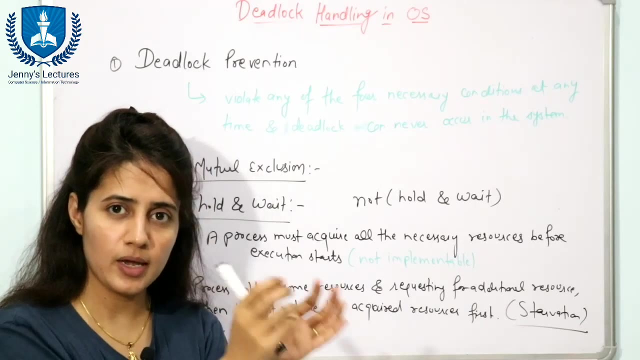 okay now. third is you allow one process is holding some resources and waiting for some other resources, but here the condition is: you, you, you just make that time bound. on the waiting time maybe suppose I have having that same example: I have having laptop, fine, and now I am holding my laptop and 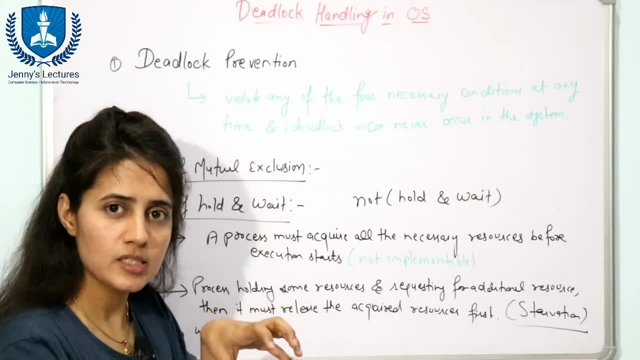 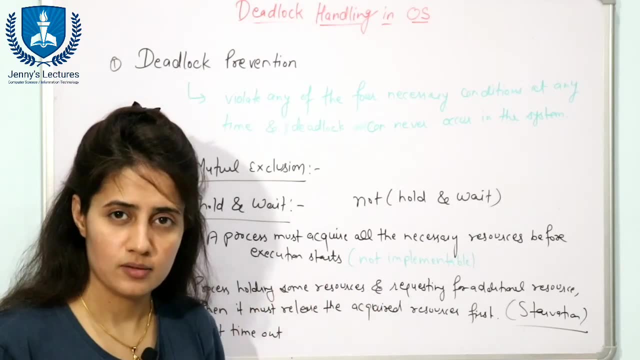 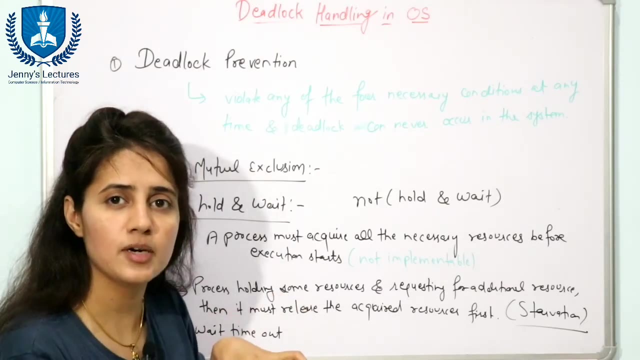 I want. I have requested for printer now. no need to release this laptop, but I can wait for printer for a limited amount of time. that is to be set and suppose that time is for that. time is 10 minutes, so I can hold that laptop and I can wait for printer for 10 minutes only if within those 10 minutes, I 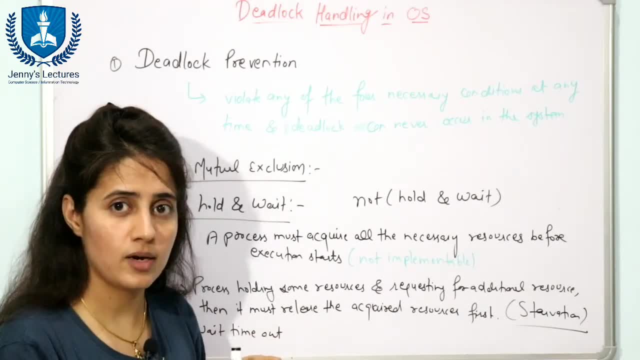 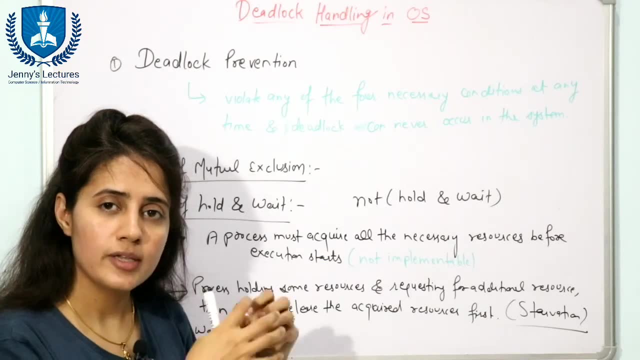 got the printer, then that is the best case. I will get the laptop also and printer also. I can do my work. but if that time bound expires, then I have to release all the acquired resources. I have to release my laptop also. fine, so there would be a time bound on the. 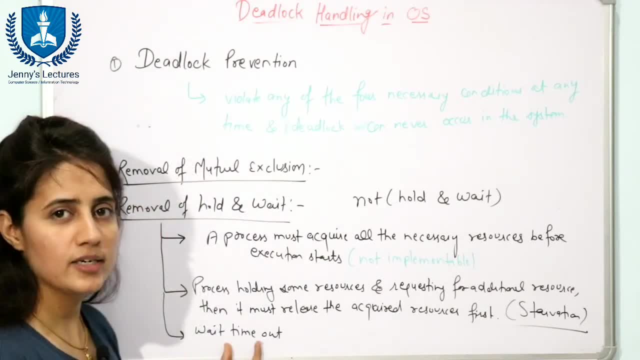 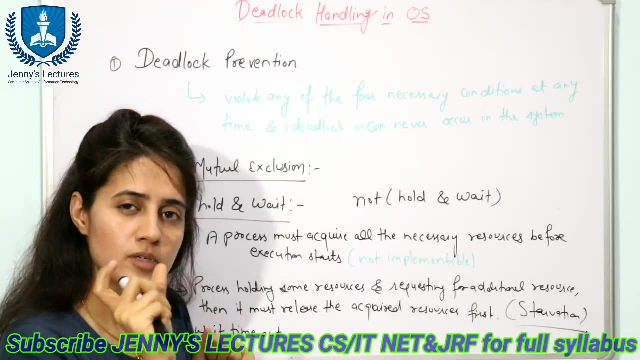 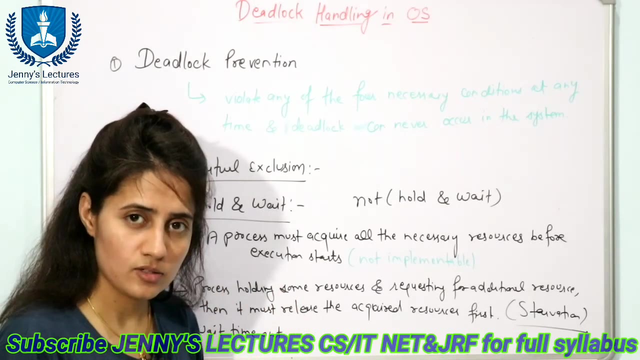 wait. that is why it is known as wait time bound. the process can hold, something can hold. some resource can wait for another resource for some time bound. if, within that time bound, that process got that resource for which it is waiting, then it is best thing. and if, but if time quantum expires. 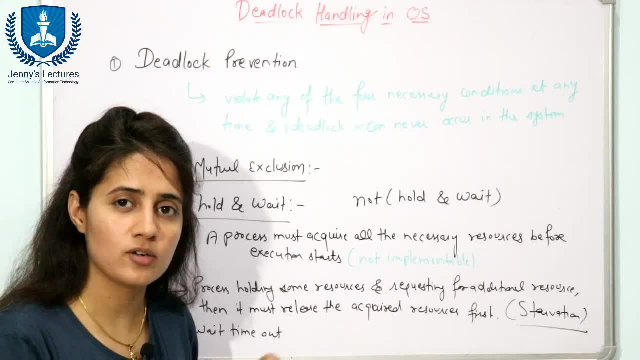 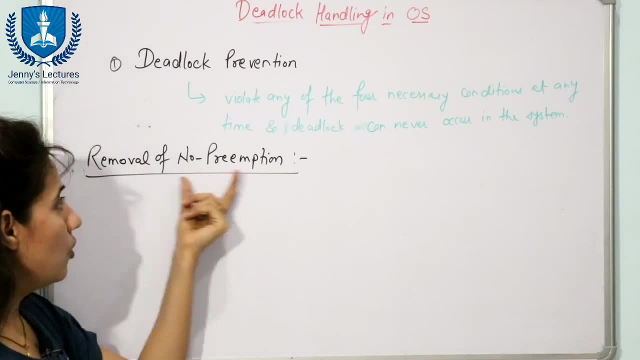 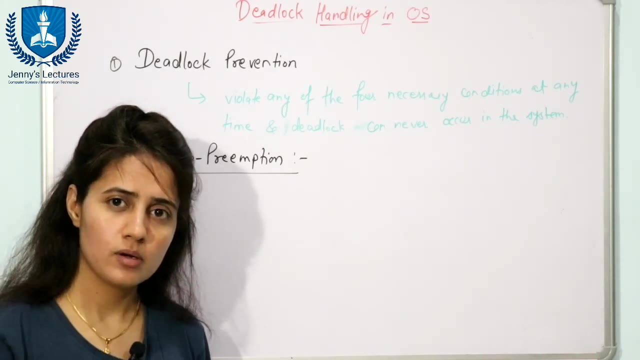 that waiting time expires, then that process has to release its acquired resources also, so that is wait time bound. so next is removal of no preemption. no preemption means you cannot forcefully take any resource from a process. fine, but now you have to remove this. no preemption means we can forcefully take. we can. 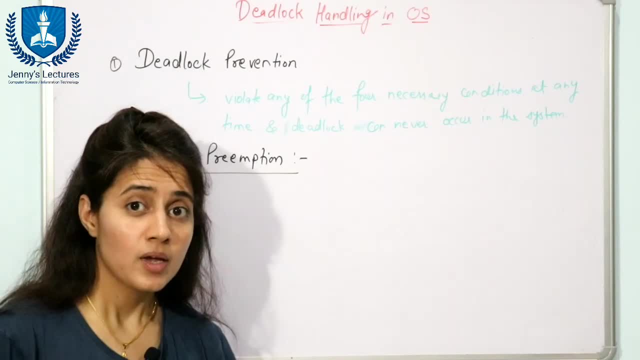 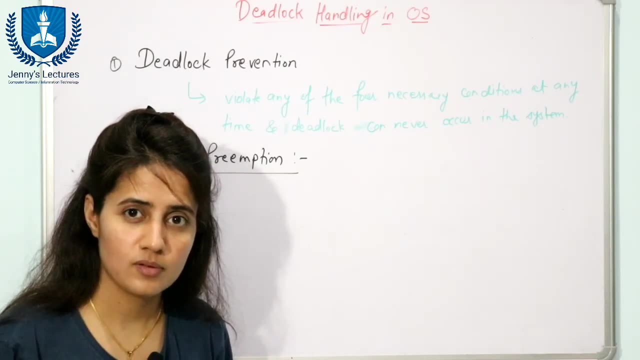 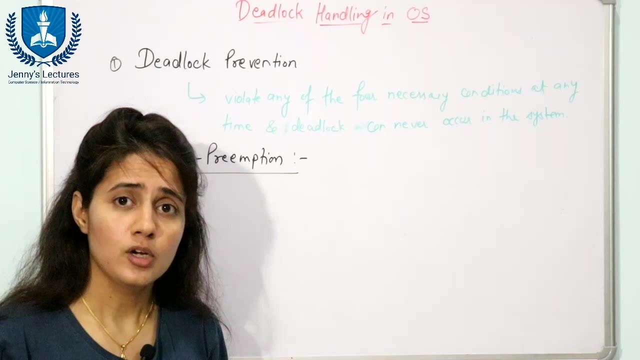 forcefully take any resource from a process, but from which process? you can take from a waiting process, not from a running process. fine, because if- and this, this kind of approach- is used by higher priority processes or you can say system processes, maybe some system process is there and that process needs some resource. fine, obviously. 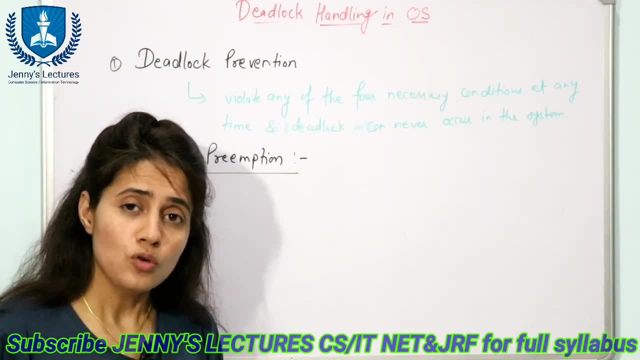 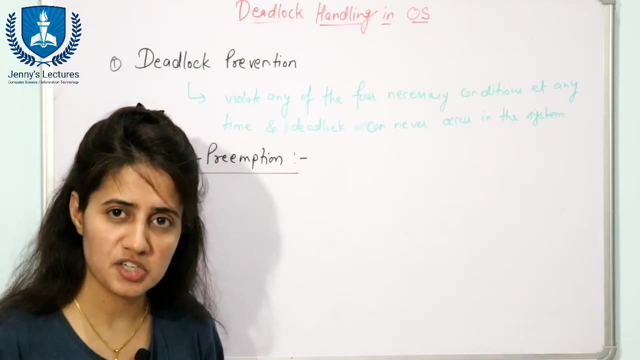 system processes having higher priority, highest priority. so we don't want that because of that resources that system process got blocked and deadlock is there. so we preempt the resource from some low priority processes and give the resources to that system process. so that is known as preemption technique. this technique is basically applied for higher priority. 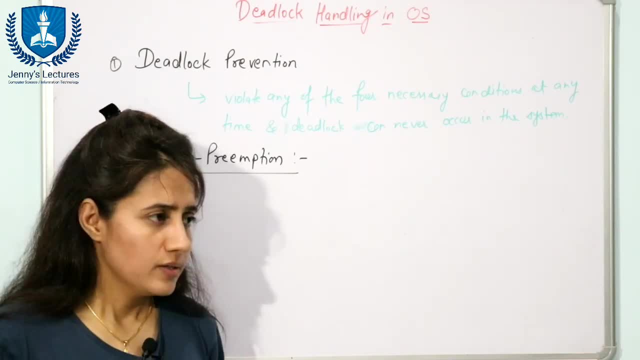 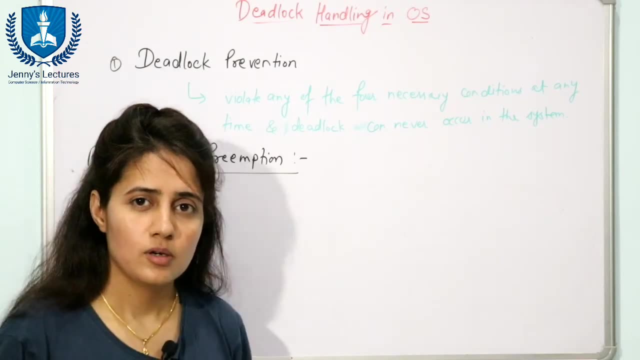 processes, or you can say system processes. let us take one example: see you, you got stuck in traffic but suddenly ambulance comes. so obviously everybody will, you know, give way to ambulance because ambulance is having higher priority. we cannot say that if we are we, we got stuck in the 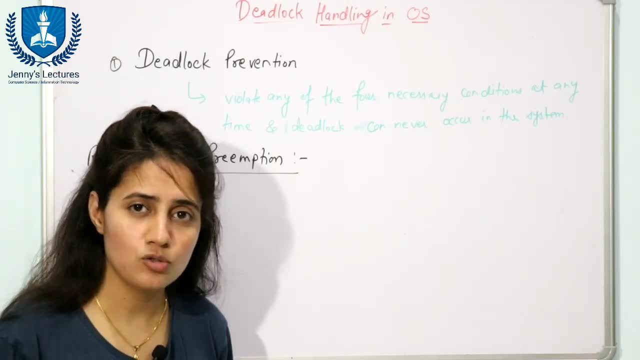 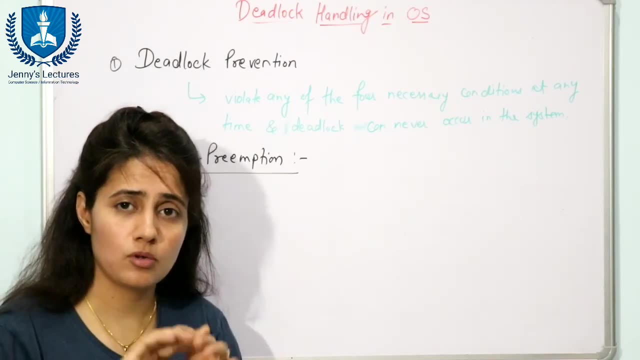 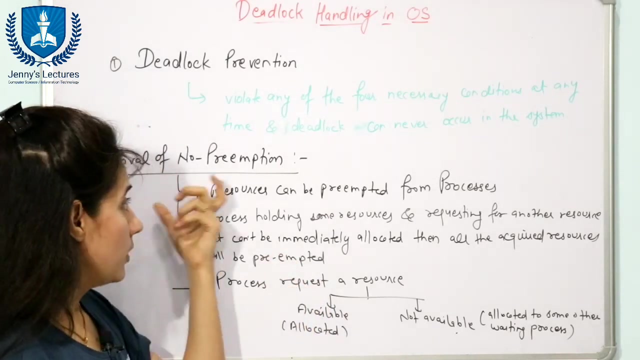 traffic, then why this ambulance is allowed to pass. that is not a case, fine. so for higher, higher priority processes this preemption technique can be applied, not for all the processes. okay, now, what is in this technique so in known preemption, in removal of non-preemption? 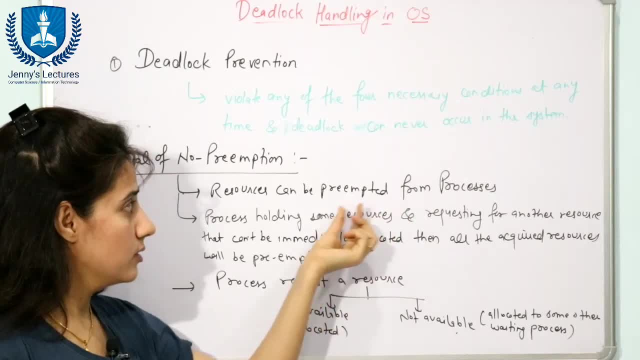 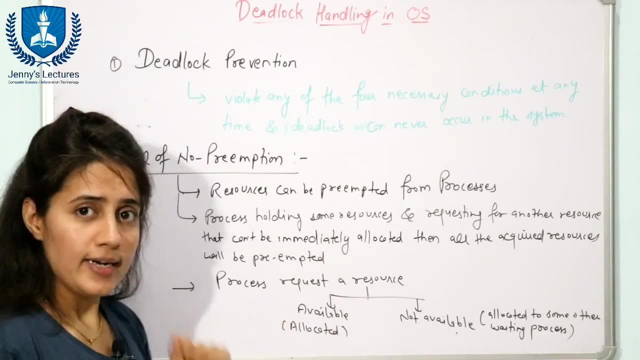 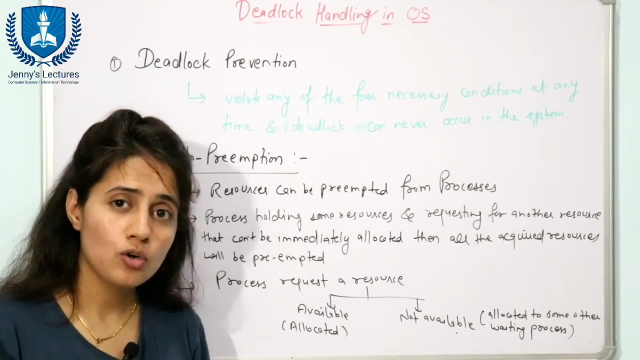 see, resources can be preempted from processes and this, this technique, will be applied for higher priority processes and you can say, for system processes. what are the techniques? one technique is if process is holding some resources and requesting some another resources but that request cannot be immediately fulfilled, we cannot give that requested resources to that. 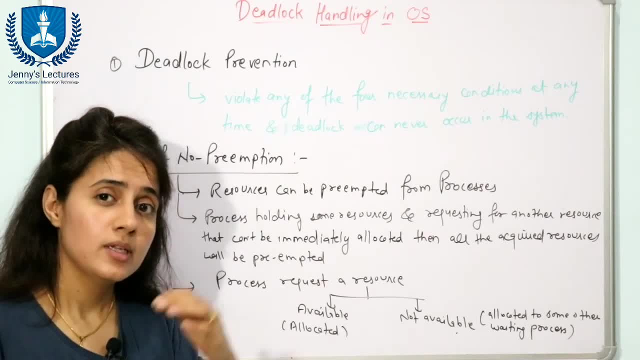 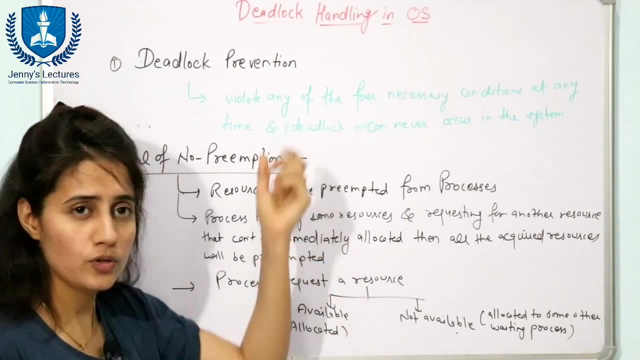 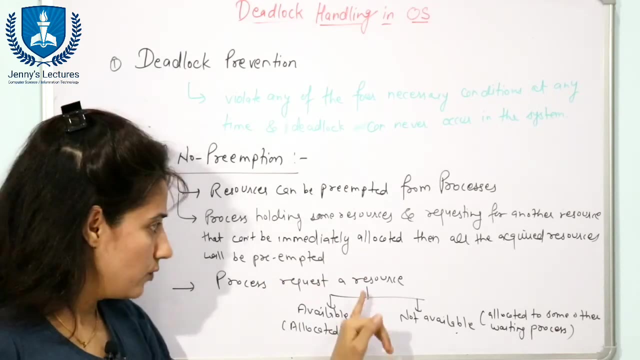 process at that particular amount of time, then what will happen then? that process, then all the resources, of all the acquired resources of that process will be preempted. same scenario which we have discussed in hold and wait. second second technique is: if suppose a process is requesting a resource, if that resource is available, then that would be allocated to that process. if that 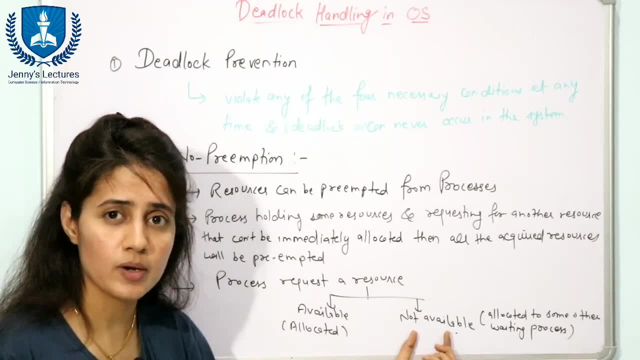 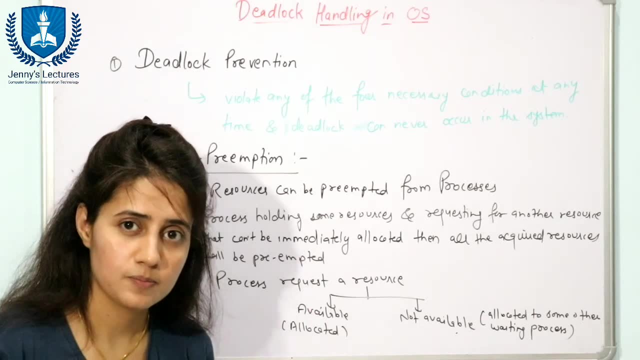 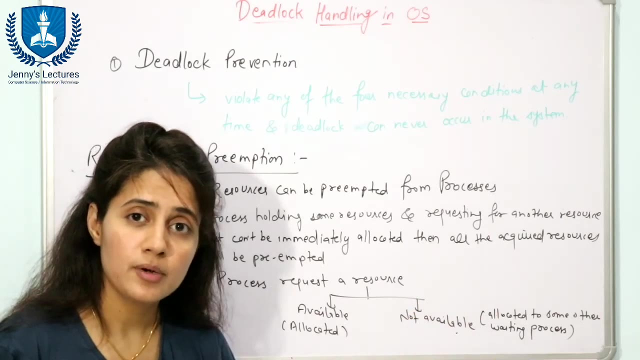 resource is not available, then we will check why this resource is not available. if that particular resource is allocated to some other process which is also in waiting state, which is also in waiting state, then what will happen? then that particular resource will be preempted from that, from that. 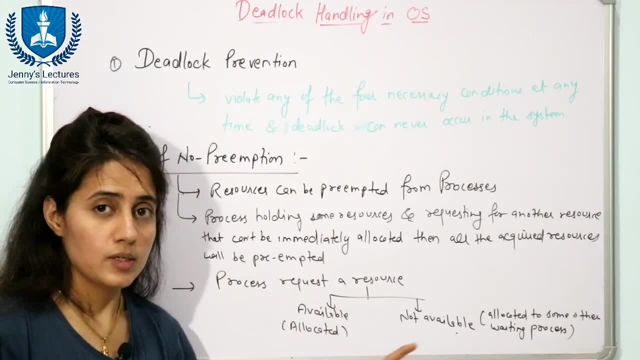 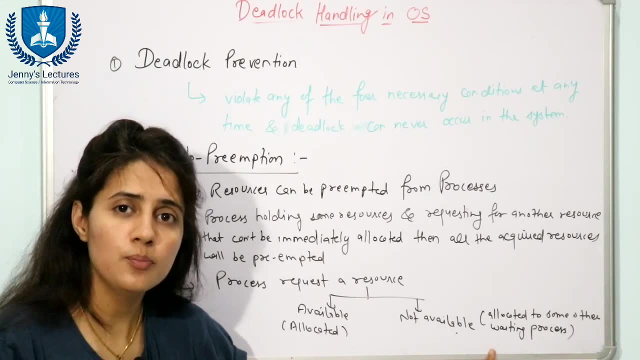 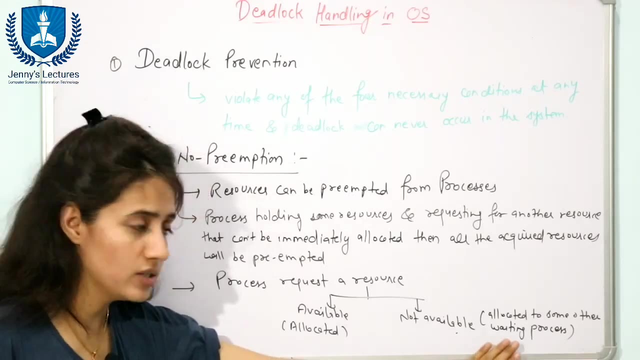 process and will be given to this process. see now here what the funda is: always the waiting process. we can only preempt resources from waiting process, not from a running process, as you can see here. see if that resource is available, then allocated. if not available, then we will check if that particular 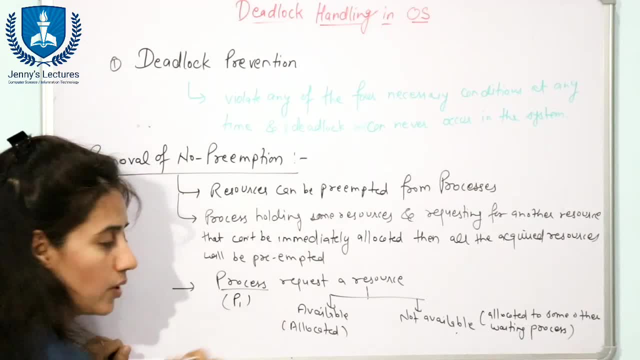 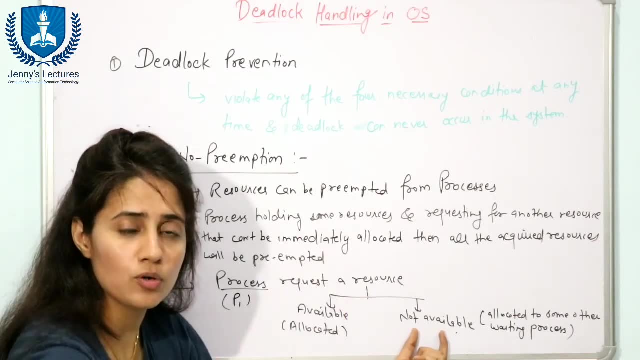 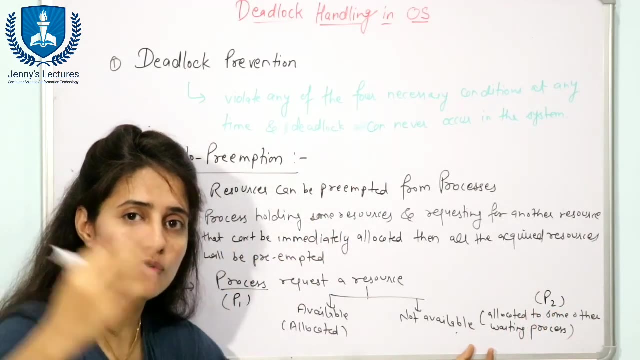 resource. suppose here is process P1. it is requesting for some resource. if this resource is not available and this resource is allocated to some other process- P2, P2 and this process is also in waiting state may be waiting for some other resource- then what we'll do? we preempt this. 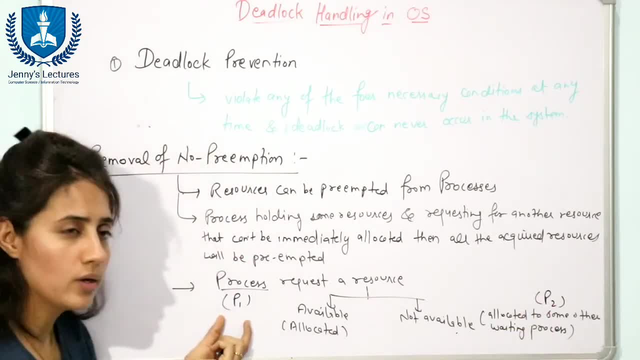 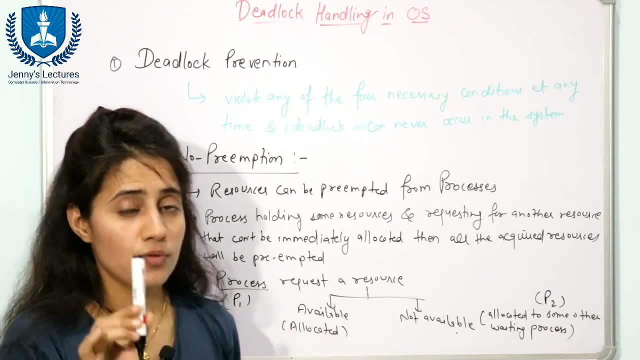 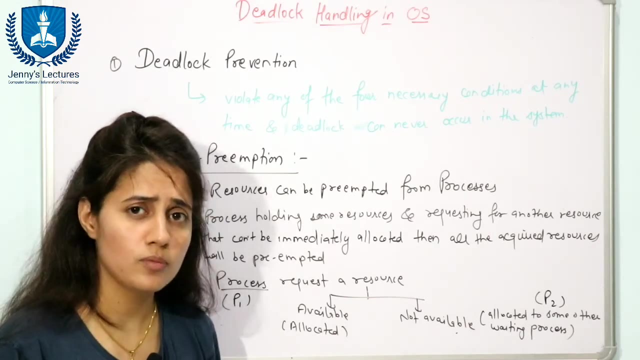 resource from P2 and this resource will be given to P1 so that P1 can do its work, its execution, fine, so make this thing very clear always: the waiting processes will be treated as victim. we can preempt resources from waiting processes from, not from running processes, fine, so this is the funda of 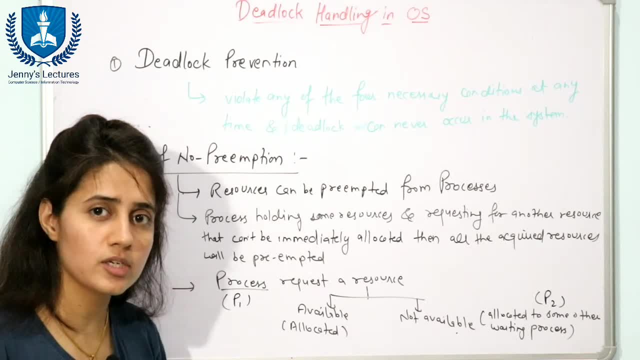 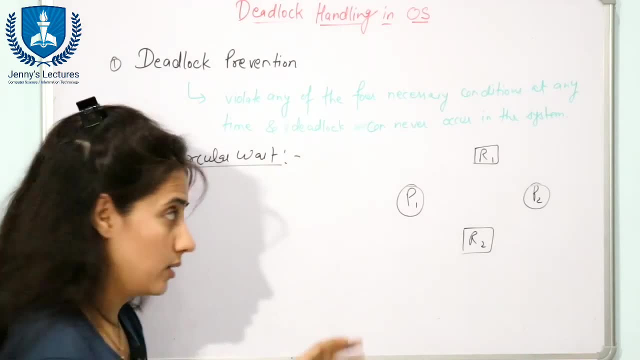 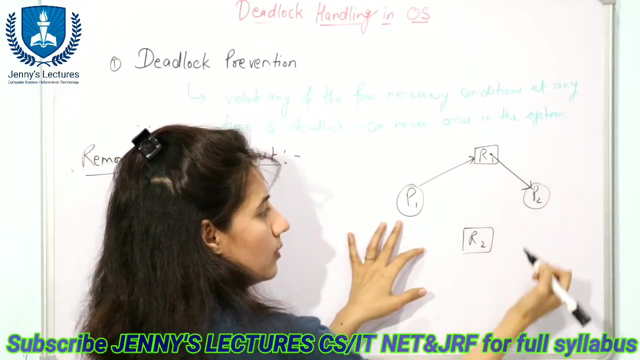 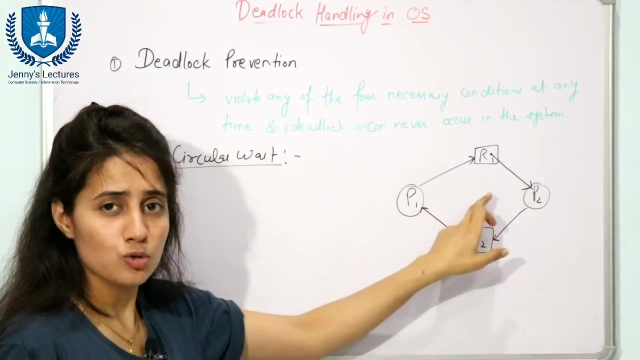 removal of no preemption technique. now the next one is removal of circular weight. see now what is the circular weight. the processes are waiting in a circle like this. suppose P1 is requesting for this R1, but R1 resources with P2. P2 is requesting for R2, but R2 is held by this P1. so this is what a circular weight. so 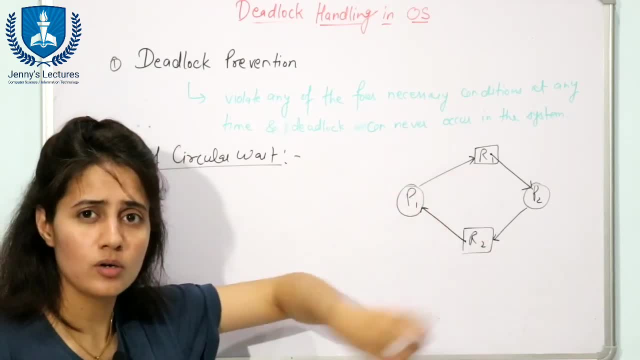 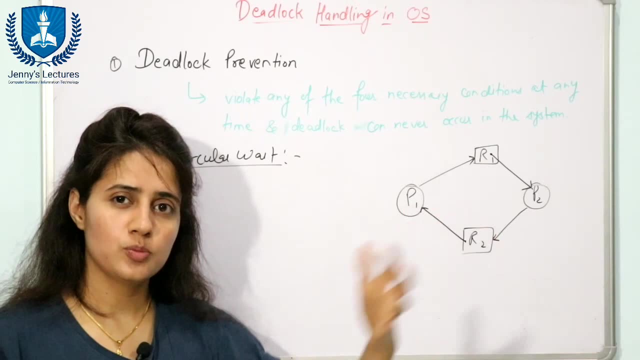 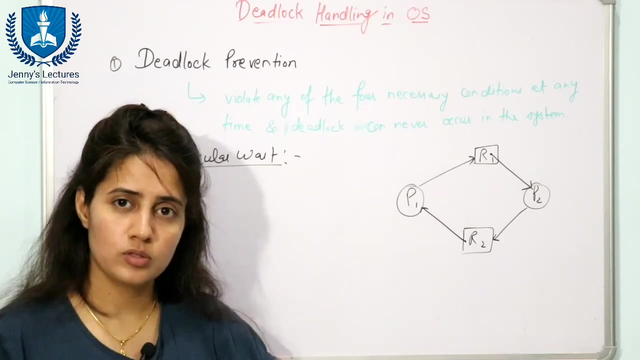 you have to remove the, the circular weight. how the circular weight can be removed, simple, funda, is: just assign a number to each process, sorry, assign an integer number to process to resources like one, two, three, four, five, like this, and after assigning the number, just make sure that the 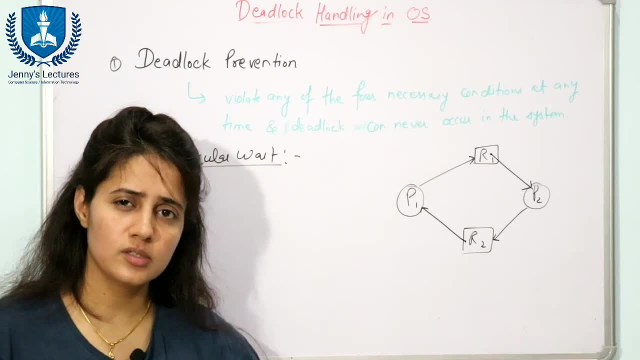 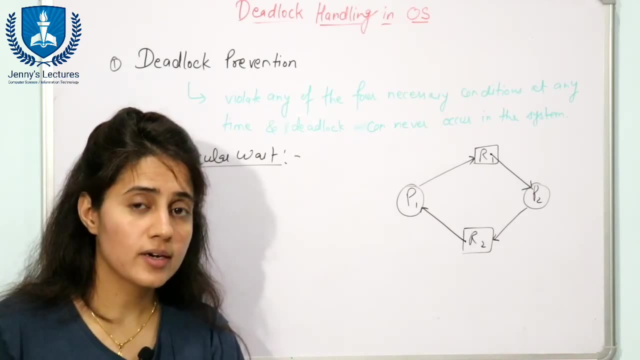 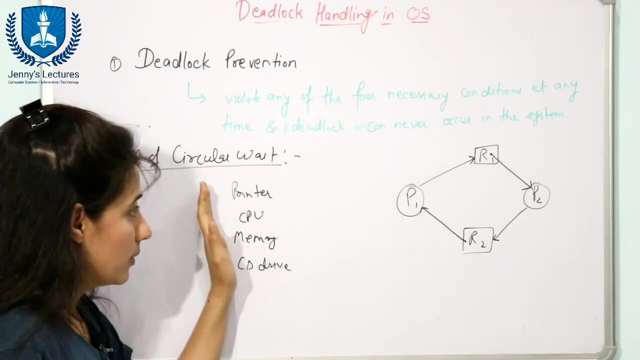 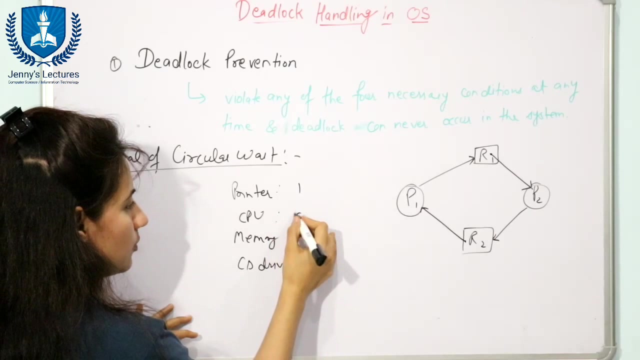 processes can request the resources in increasing order only or decreasing order, strictly increasing or strictly decreasing order only. see, let us take this example, these are some resources, so some numerical, some numerical integer value will be assigned to these. so resources like one, suppose five, suppose six, suppose seven, now suppose two processes are there. 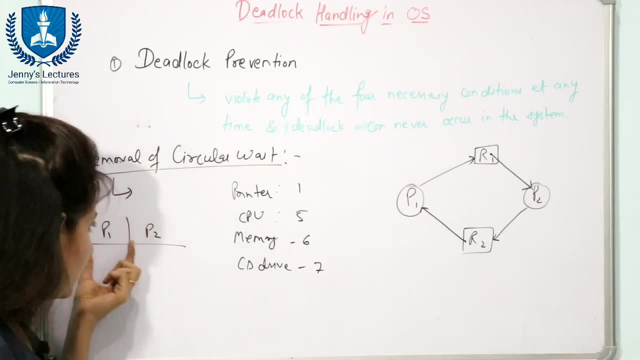 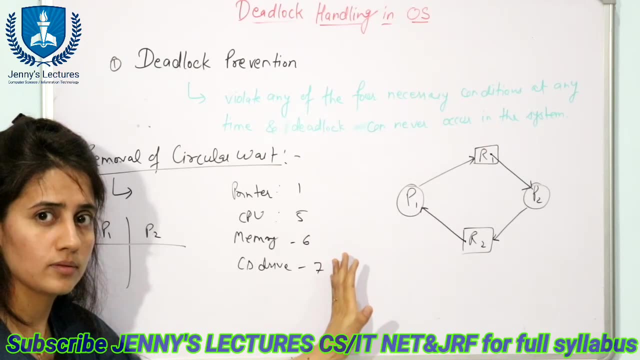 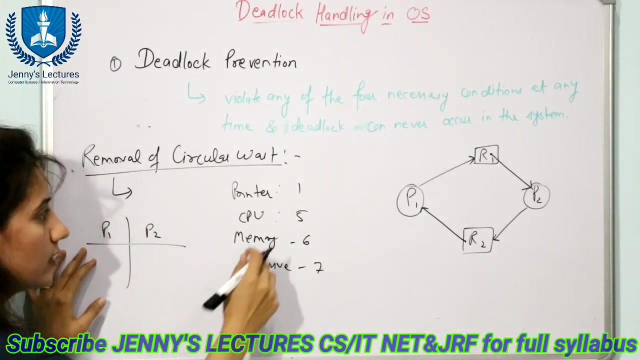 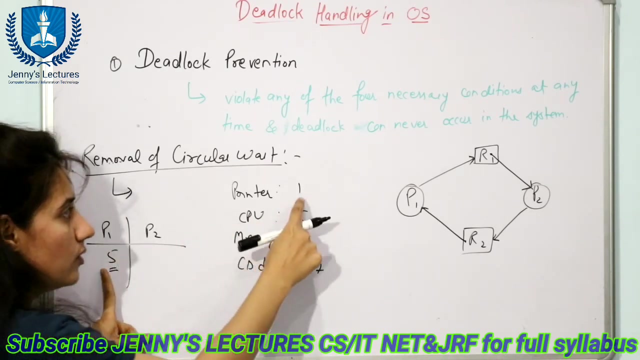 P1 and P2. now, these P1 and P2 processes can only request the resources, only in its increasing order. fine, like one, five, six and seven, like some particular amount of time, P1 is, P1 is holding a resource having number five, that is, CPU. and now P1 is requesting for this printer. 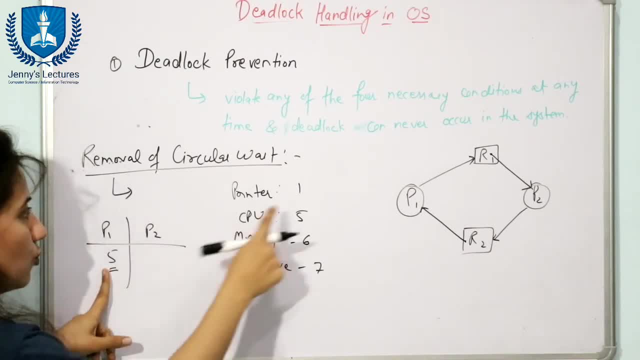 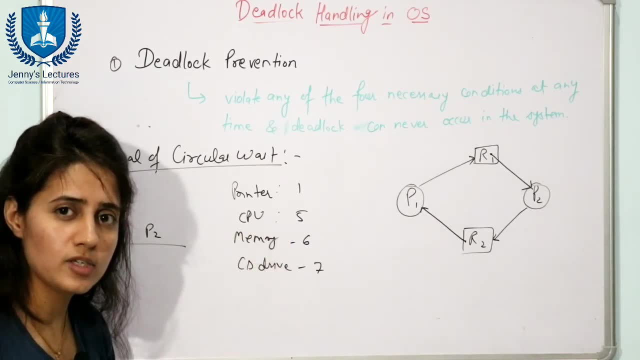 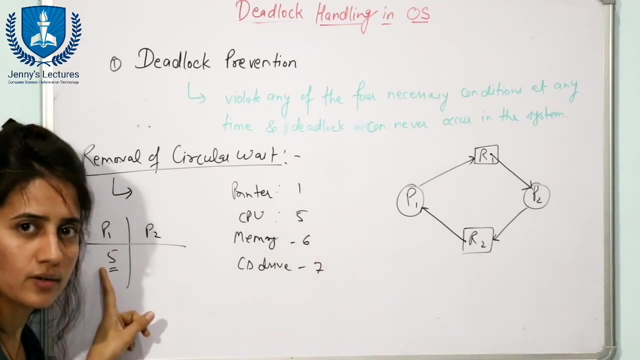 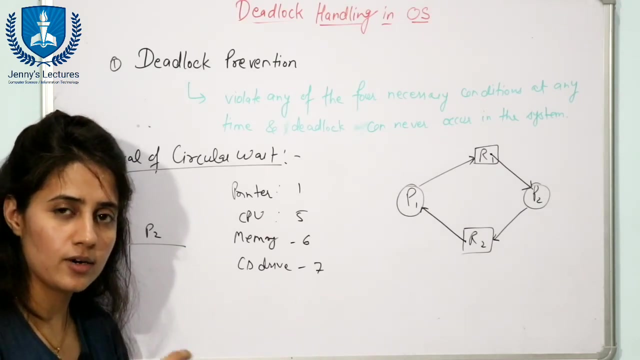 is it possible? no, that would not be possible, because one one is less than five. if the algorithm is like that the resources can be requested in increasing order, then what? what would be the case? P1 can request only six and seven. P1 cannot request one. if the algorithm is applied something like this, that processes can request the. 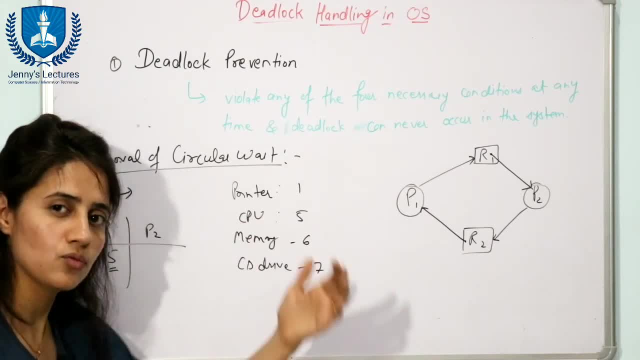 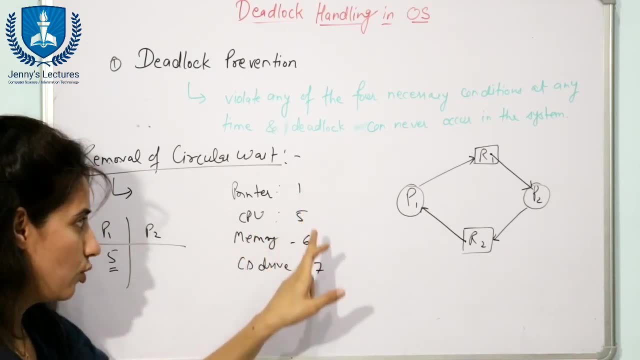 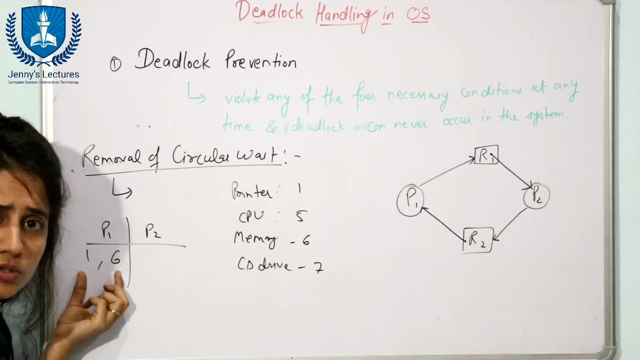 resources in strictly decreasing order, then what will happen? then? vice versa won't be there. then what will happen? if it is having five, then it can request only this one. it cannot request six and seven. now one case is there: for that particular amount of time, P1 is holding a resource number one. 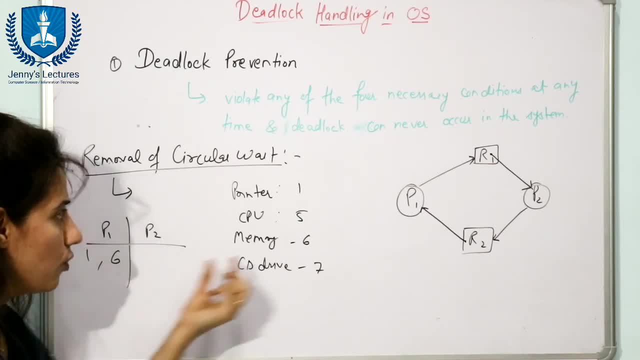 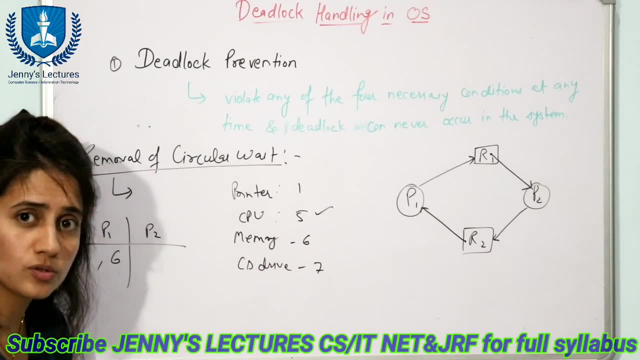 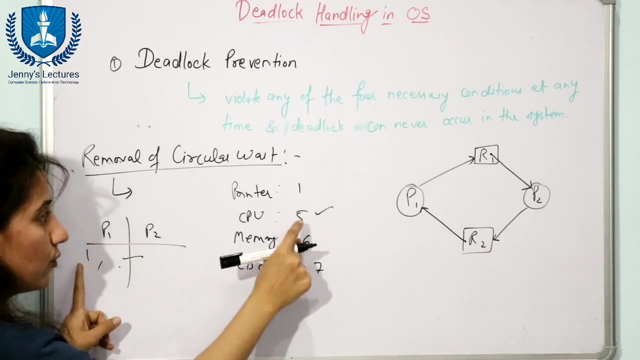 6. fine. now p1 wants this 5 resource. then what will happen? it cannot request this 5 resource. then what the alternative approach is? what this p1 would release would release the resource 6- fine, and now p1 can request this resource 5, and again for 6. this is the case, so simply, you can. 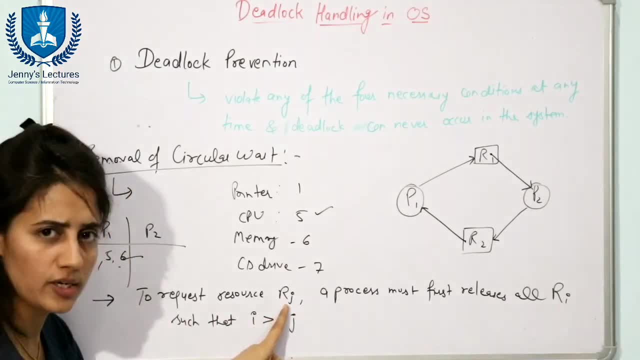 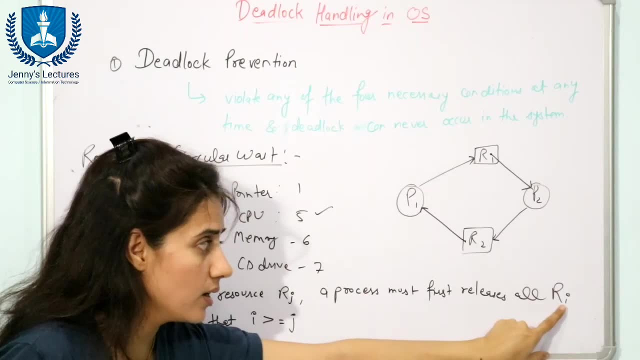 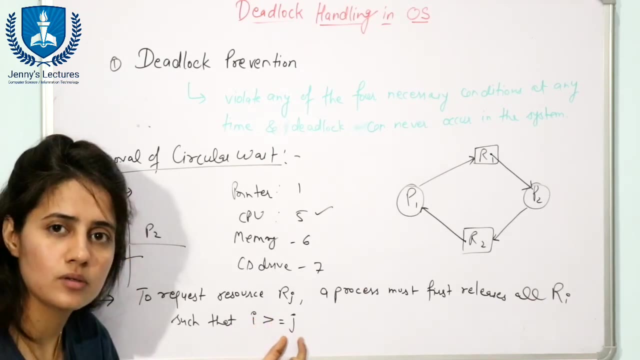 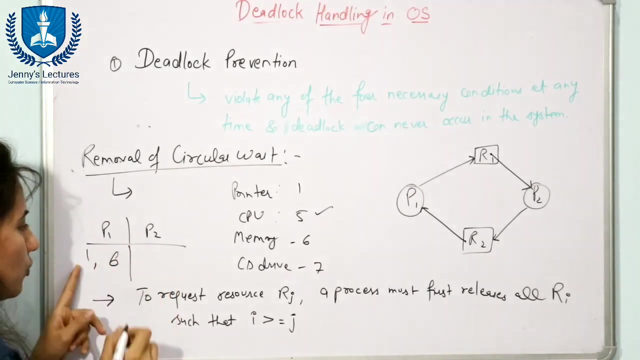 write to request a resource. suppose rj, rj. a process must first release all the acquired resources: r i, r? i such that such that i is greater than or equal to j? r? i such that such that i is greater than or equal to j. here you can say, here just, we can just take one case: p1 is holding 1 and 6. now p1 is requesting for. 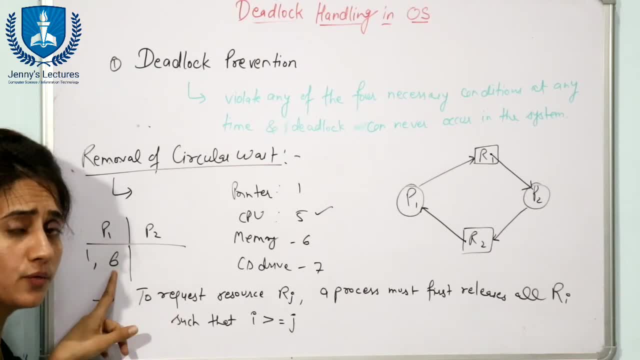 this 5, then p1 has to release this 6, because i here, i is what- 6. so p1 has to release this 6 because 6 is greater than equal to this. j fine, after that it can request this 5 and then can. 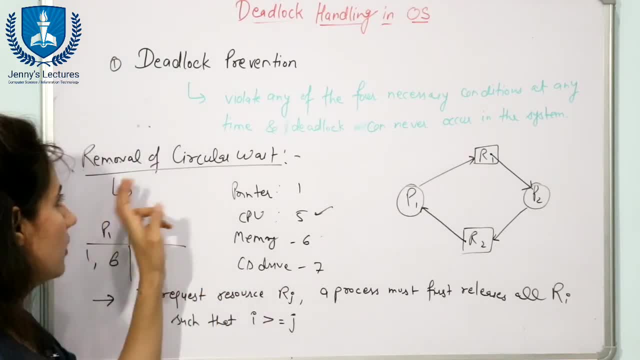 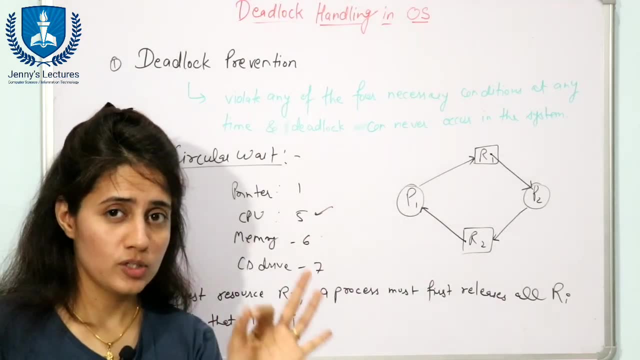 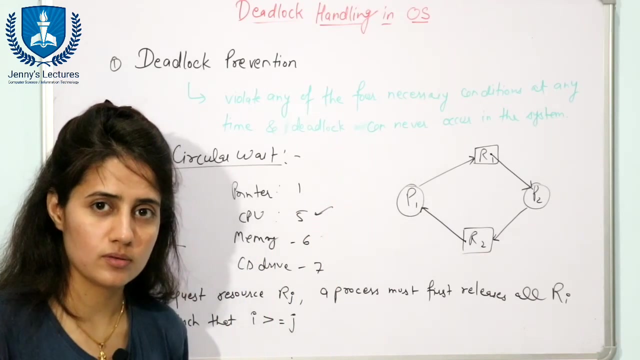 request to 6. so this is how you can. you can implement this removal of circular weight. just make sure that processes can request the resources in either strictly increasing order or in strictly decreasing order, and every resource is assigned some number. so here problem of in implementation of this. 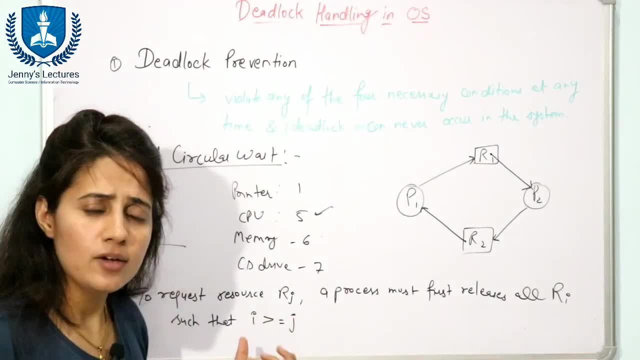 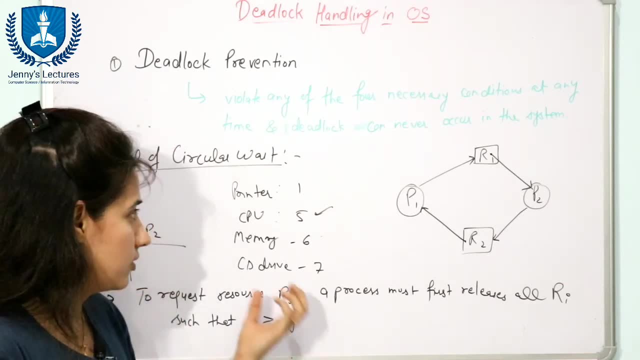 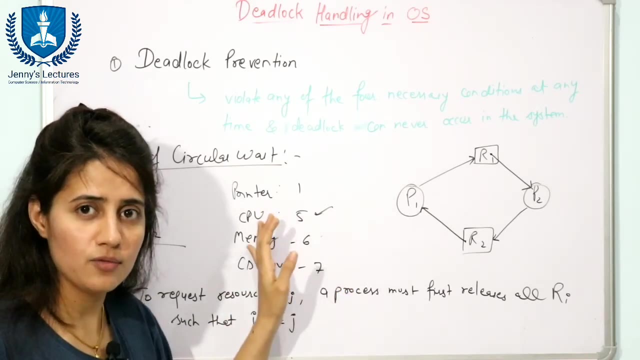 technique is what see? it is very difficult to determine the relative ordering of different resources. many resources are not able to determine the relative ordering of different resources. so how to how to determine the, you know, the relative ordering of these resources. so that is very tough, although it is implementable, we can implement. we can remove the circular weight, just assign a number. 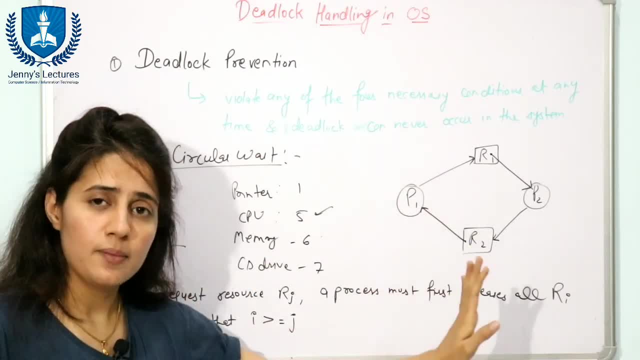 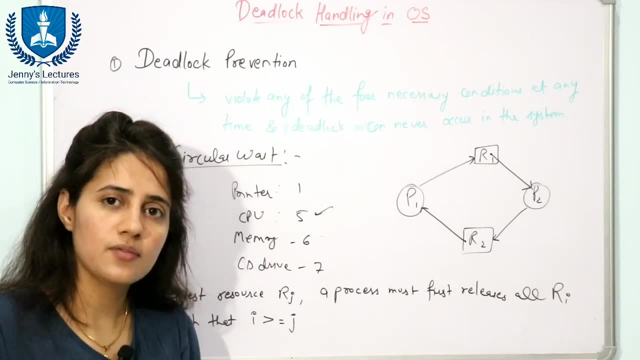 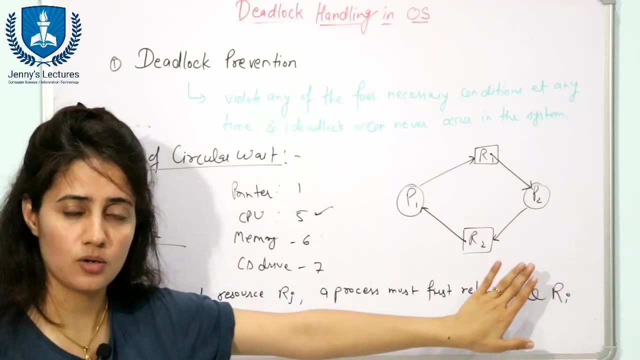 numeric integer or you can say priority to each resource and make sure that processes can only request the resources in increasing order, strictly increasing order or strictly decreasing order. then there would not be circular weight. never there would be circular weight. let us take this example: only see at some particular point of time. 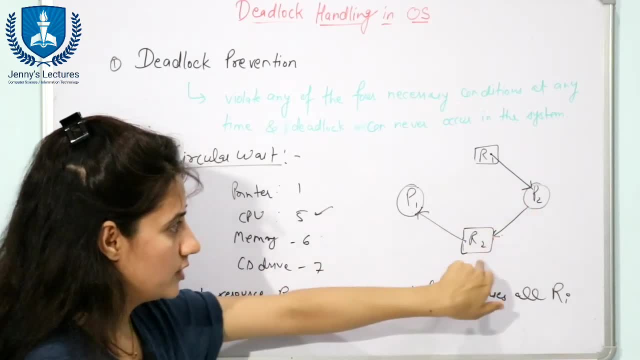 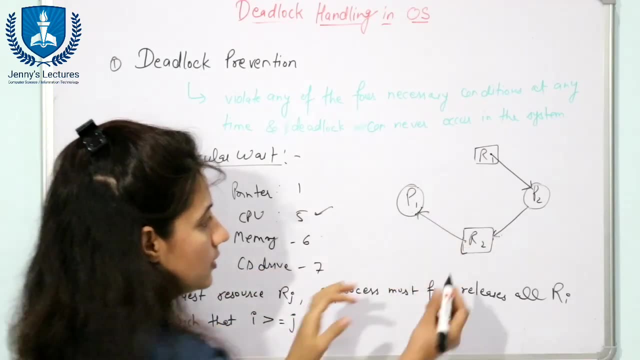 this: p2 is holding r1 and p2 is requesting r2. p2 can request r2 because it can request all the resources greater than 1, 2, 3, 4, 5, like this: and this: suppose r2, r2 is with p1, suppose p1 is holding: 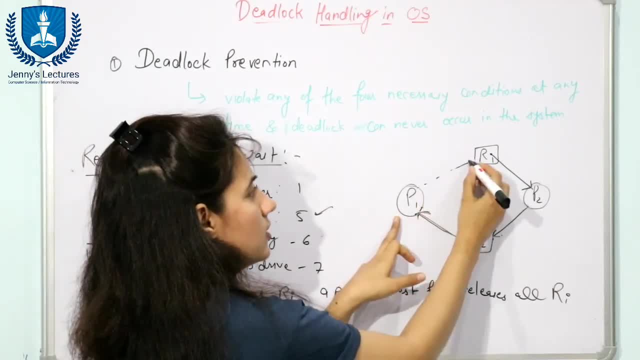 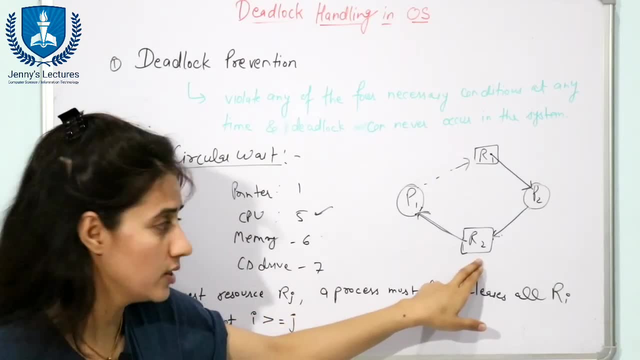 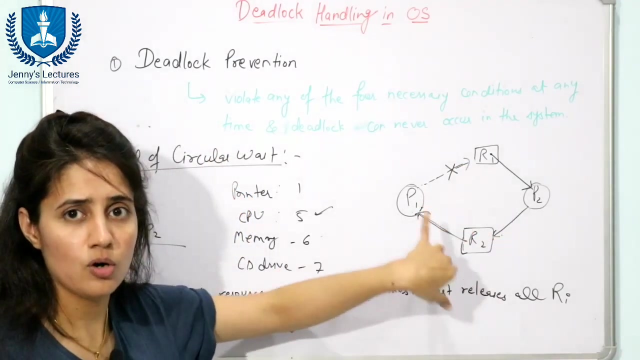 this r2. now. can p1, p1 request this r1? no, why so? because p1 is holding this r2 and p2 is requesting are two, so we can. it cannot request any resource less than two, so that is why we cannot put this edge. if you will not put this edge, then there will not be. 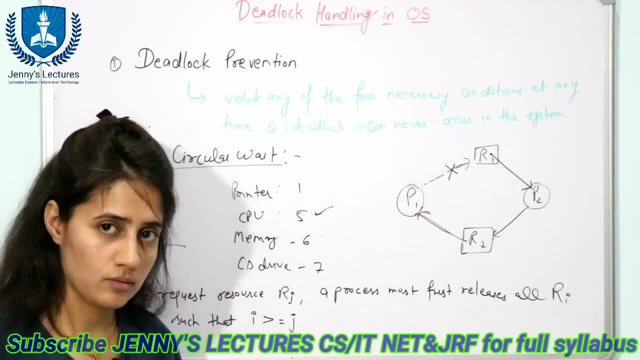 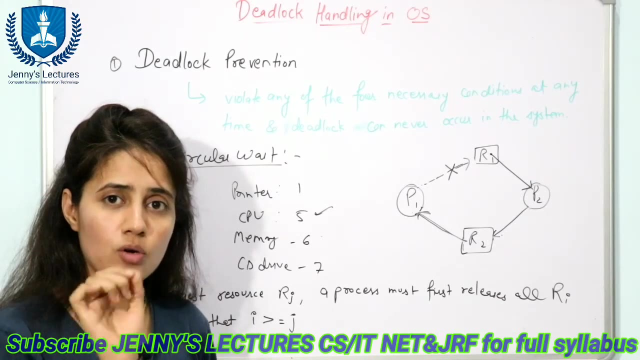 circular weight. so you can take any other example. if this kind of thing- total ordering- is there, then there would not be circular weight, definitely so. this is all the deadlock of all about deadlock prevention techniques. in next video we will discuss deadlock avoidance technique. or you can say bankers. algorithm. till then bye, bye, take care.